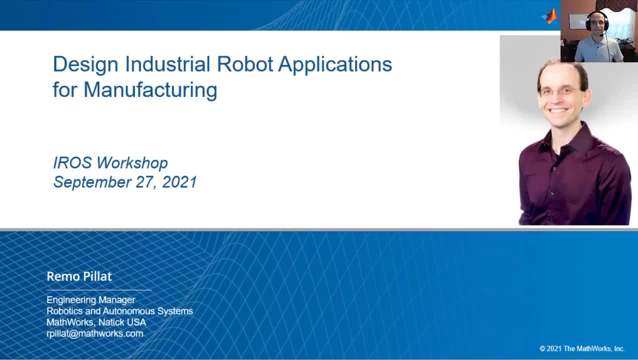 Hi, my name is Remo Pillert and I'm an engineering manager at MathWorks working on several software products for robotics and autonomous systems. As part of our development work, we interact a lot with industrial robotics companies and we see some clear market trends that I would like to share with you today and summarize how these market trends impose requirements on the software development process. 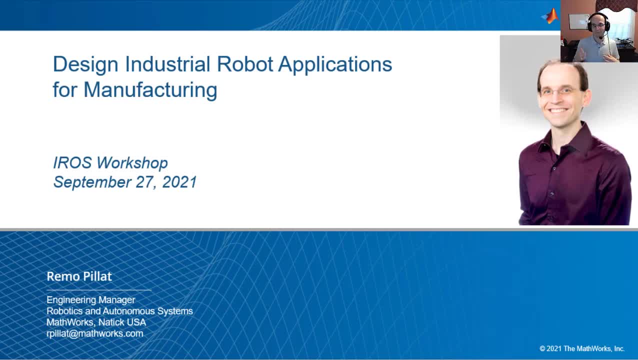 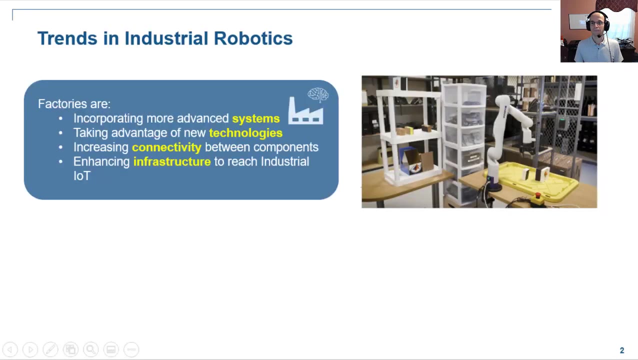 Full disclosure. since I'm at MathWorks, some of my slides will focus on how MATLAB and Simulink can be used for this application space, But I believe that a lot of the basic development process translates to other tools as well, So let's get started. 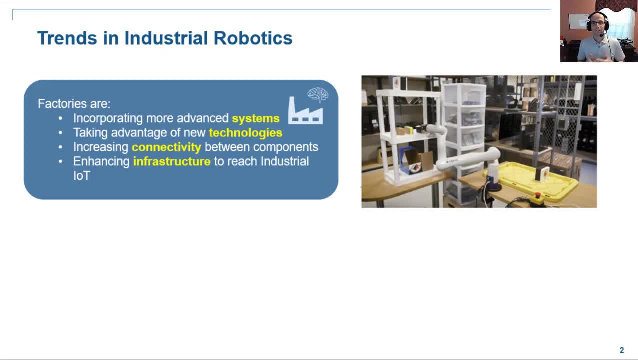 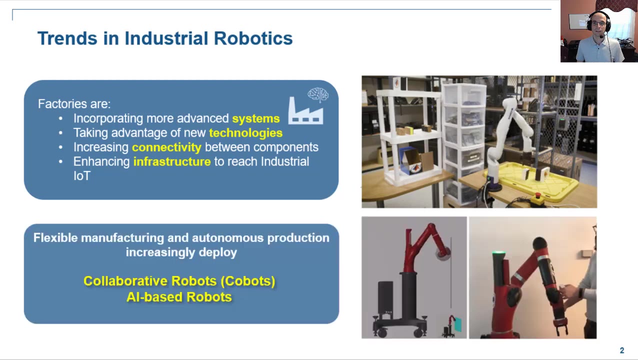 Let me start with some industrial robotics trends. The digital technology development is now enabling a new wave on manufacturing innovation, And factory factories are incorporating more advanced systems and taking advantage of new technology. Specifically, factories are now combining advanced systems like collaborative robots and AI-based robots to get work done. 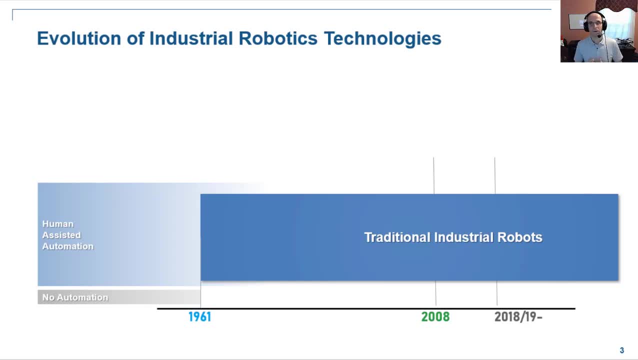 And this exciting robot trend really follows many decades of deploying traditional industrial robots. The first one of those was actually deployed by General Motors in 1961. There wasn't much fanfare about it and American companies didn't really use industrial robots for quite a while after that. 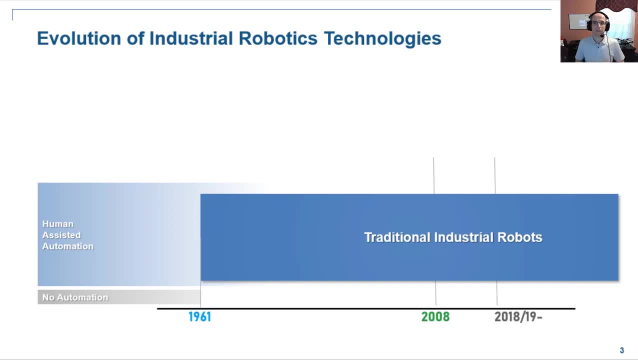 But these traditional industrial robots really focused on automation and mass production and typically just follow a predefined path. Those robots also have to be fenced in for human safety. Around 15 years ago, collaborative robots, or co-bots, first entered the market, Working alongside humans. 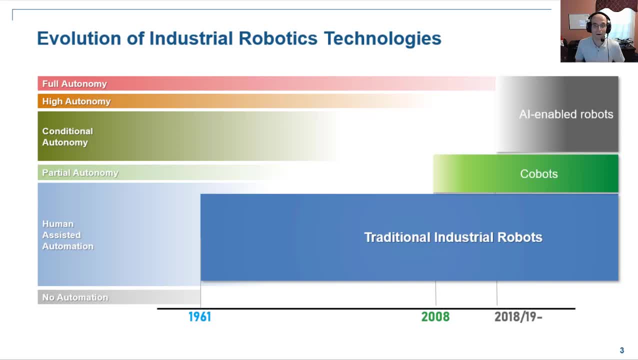 co-bots had to be safe and employ a new level of autonomy to ensure that safety. One of the entrants back then was Universal Robots in 2008.. They are now the market leader for co-bots and sell more than 50% of all co-bots on the market. 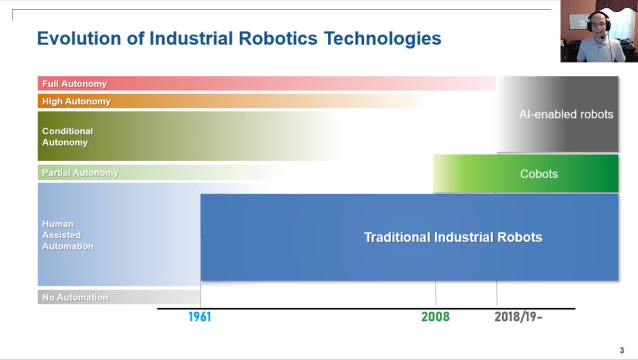 More recently, AI-enabled robots reached new heights for autonomy, But these are mostly relegated to the R&D domain. These robots are now more and more popular, But the overarching trend here that I want to highlight is that manufacturing is going from mass production to mass customization. 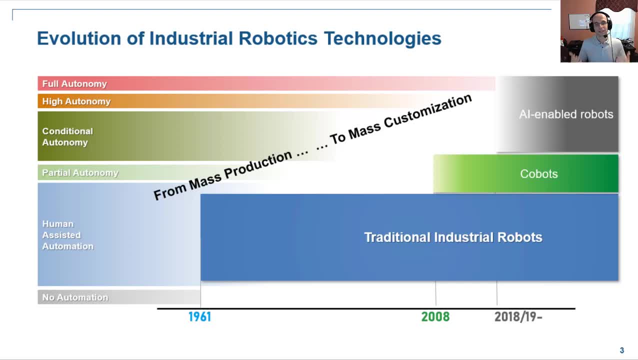 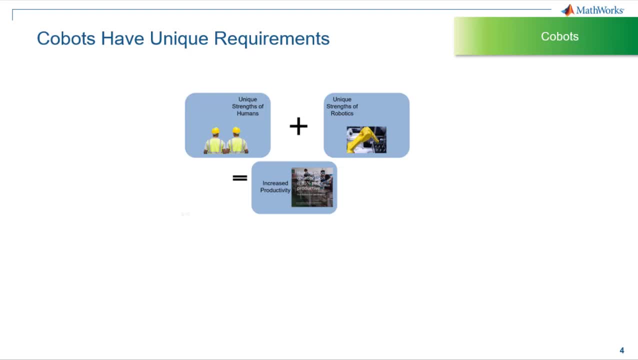 Because more intelligence in robots means more customization of the manufacturing process. So I want to focus on these co-bots again, since they are just at this threshold of becoming, of being economically viable and being deployed right now. So I want to focus on these co-bots again, since they are just at this threshold of becoming 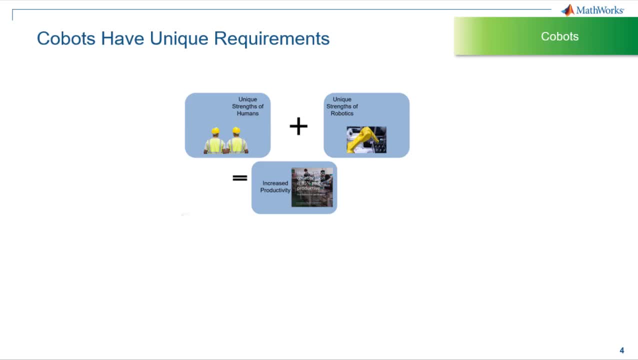 And if it turns out that more intelligence is required, it means more dzisiaj a jobs, as these mounted robots can that and what's hard to find and what could be teached worldwide. So co-bots impose unique requirements, since they share workspace with humans. 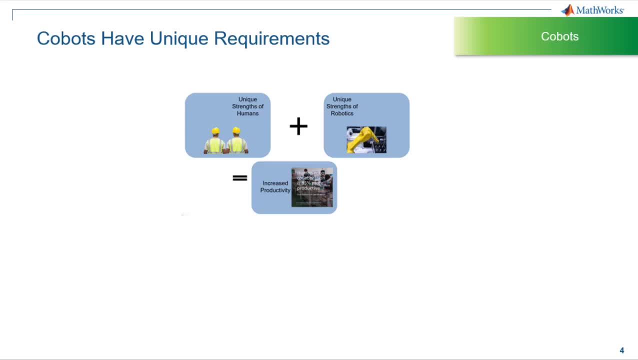 So co-bots impose unique requirements, since they share workspace with humans, and that requires them to have a certain level of autonomy for ensuring worker safety, and that requires them to have a certain level of autonomy for ensuring worker safety. They also operate in an environment that is both dynamic and unpredictable. 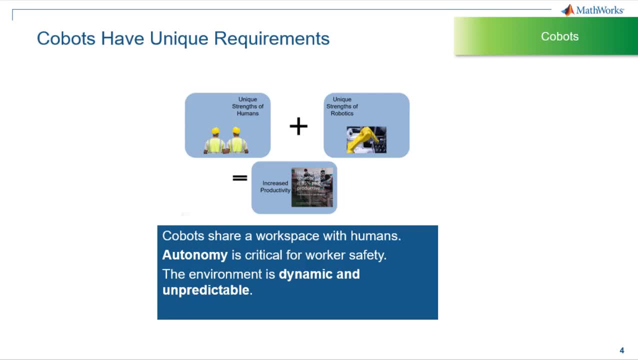 So none of these cages of the traditional robots I've called co-bots anymore. So none of these cages of the traditional robots I've called co-bots anymore. So none of these cages of the traditional robots I've called co-bots anymore. 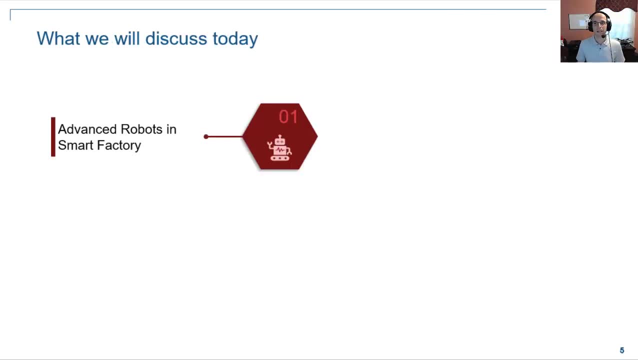 So what we'll discuss today in my talk is I'll begin giving some context about the place and in which this동 걸�beack gives up a sense of the Turks. What we'll discuss today in my talk is I'll begin giving some context about the place. 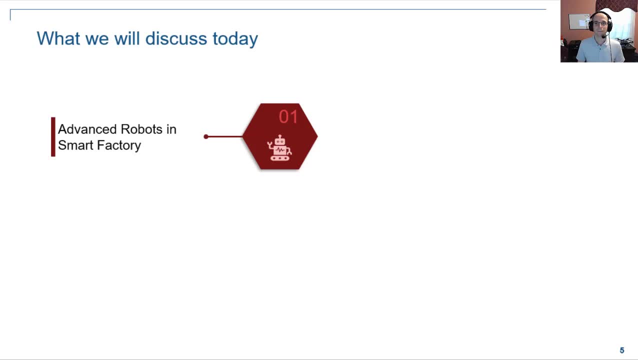 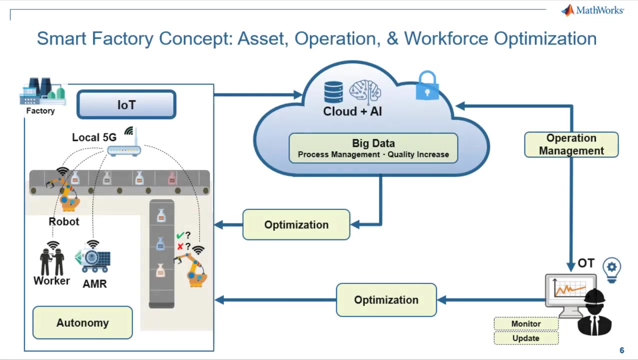 of smart robots in the factory and then talk about how we can develop autonomous robotic systems, and I'm going to show a particular application. pick and place has been popular for many decades now, but it's still a task that has to be performed regularly. and finally, I will summarize what I showed. 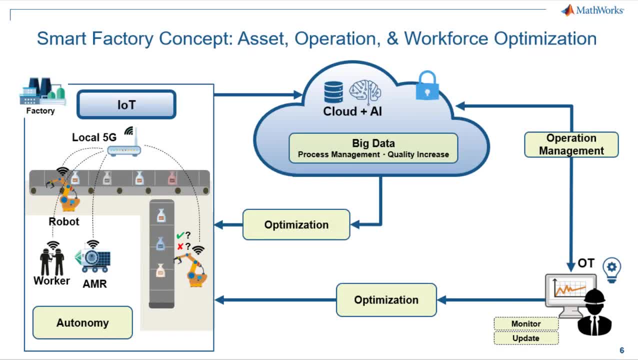 So in recent years, with the introduction of more digital tools, the smart factory concept has been promoted in manufacturing systems, and there are lots of parts to the smart factory, but one of the important one is that data collection happens all across the factory through IoT devices or other sensors in the environment. 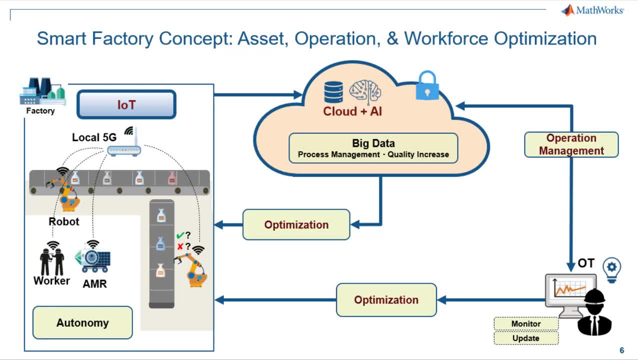 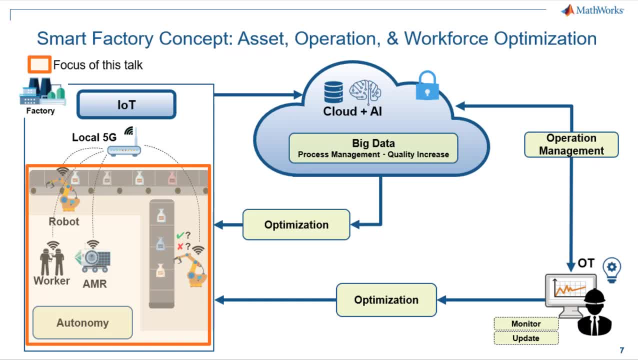 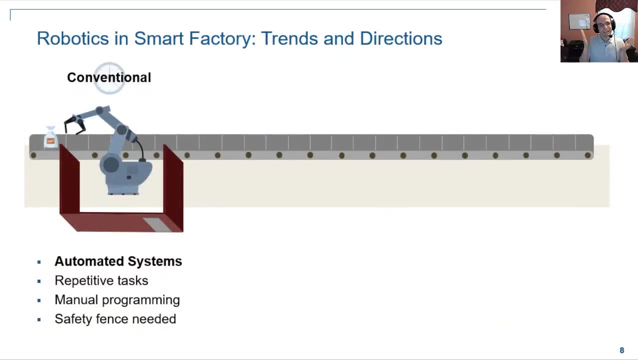 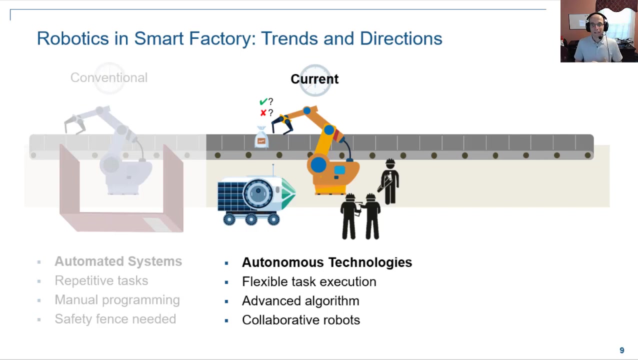 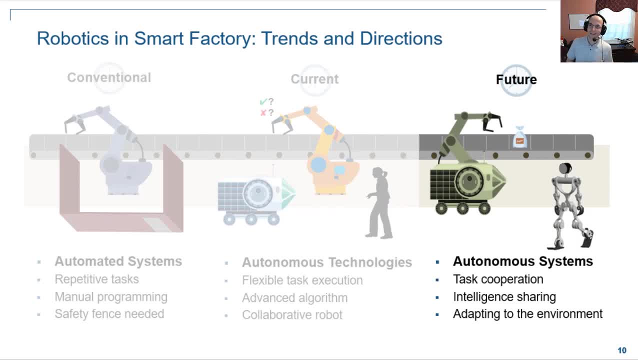 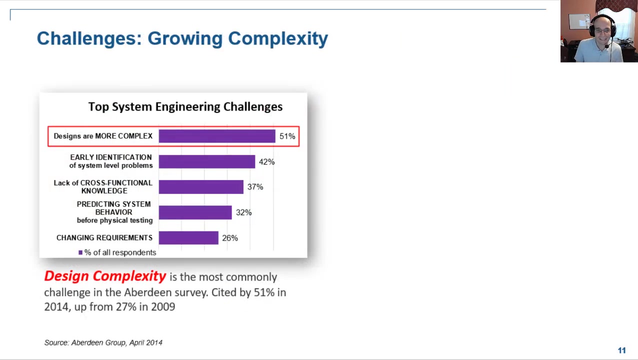 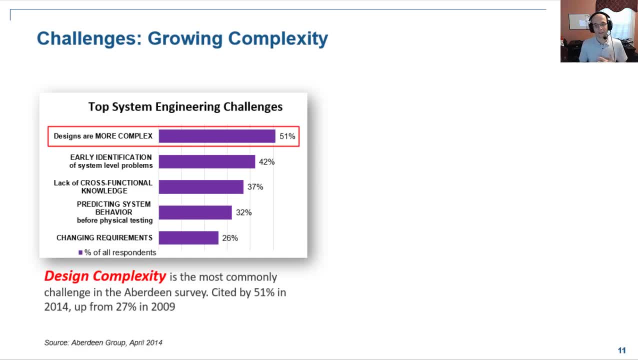 and these new cobots in the industrial space. So what we hear a lot from customers and from industrial robot companies is that the designs for these robots are getting more complex, And that's the top engineering challenge, because all this autonomy has to be built and all this autonomy. 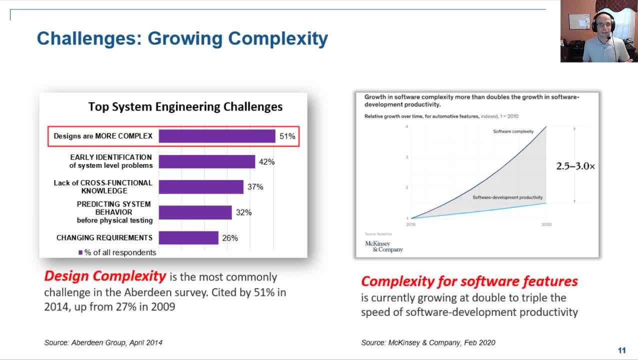 is taking place, typically based around software, And software complexity has been increasing for a while now, whereas the ability for our software developers to develop that software has increased more linearly. So how do you manage all this complexity that's needed for this autonomy on the factory floor? 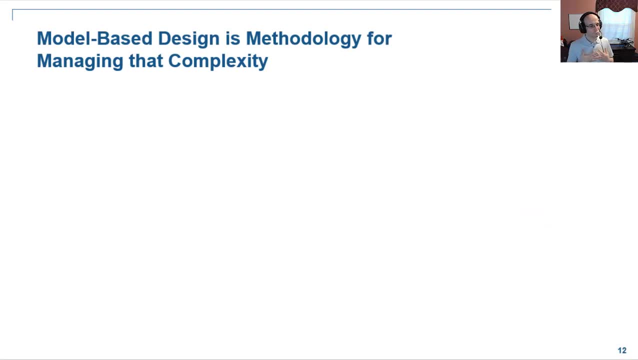 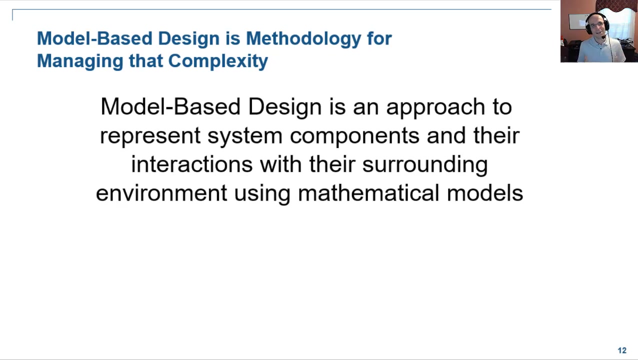 Well, one way to do this that I see, and I happen to think is a good way, is using model based design and really using that as a driving methodology for managing the complexity. So what is model based design? Well, the raw definition is that model based design. 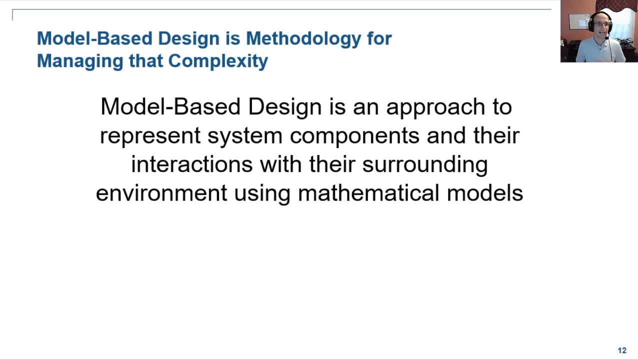 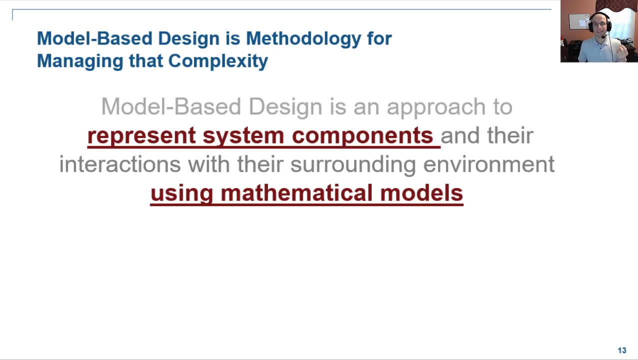 is an approach to representing system components and their interactions with their surrounding environment using mathematical models. It's a bit of a mouthful, but the two key pieces here is that you're representing parts of the system as modules and that you use math and simulation. 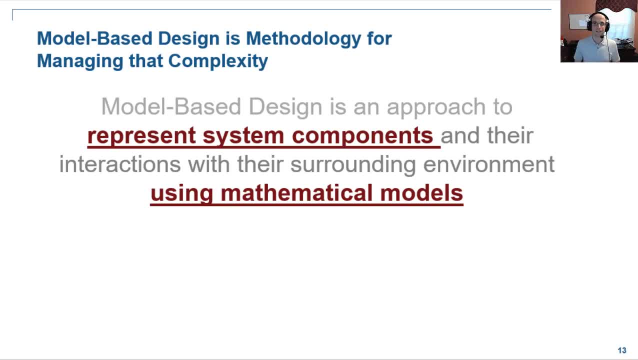 to validate these models. So who uses model based design? Well, it turns out most of the automotive and aerospace companies in the world adopt that model based design for designing their systems, So it seems natural to also apply that same methodology to industrial robots. 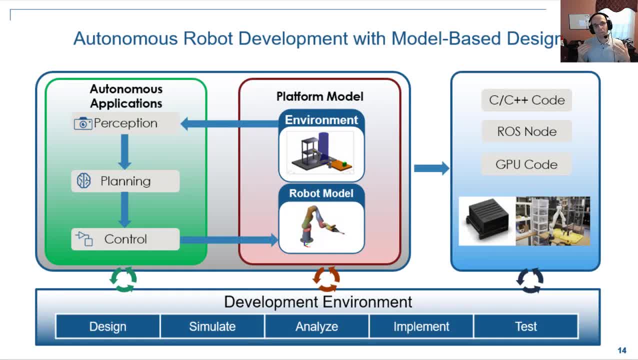 And that's what I wanna dig a little bit into, Like what would model based design look like for industrial robotics? So there are really like a common set of workflows that you will encounter when you design a robot application, And it really has three pillars. 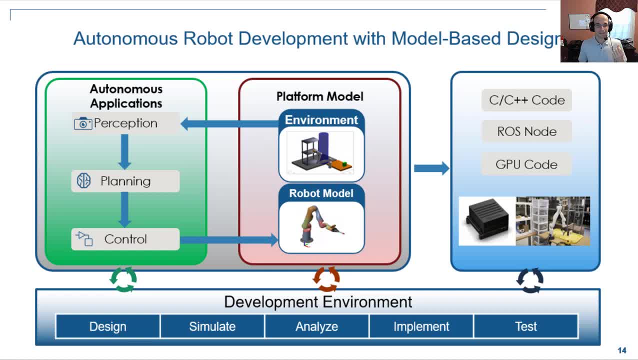 One is designing the platform and its environment that it needs to interact with, Then building some software and technology to use it, Then building some software and technology on top of that platform- Things for things like perception, planning and control- And, in the end, 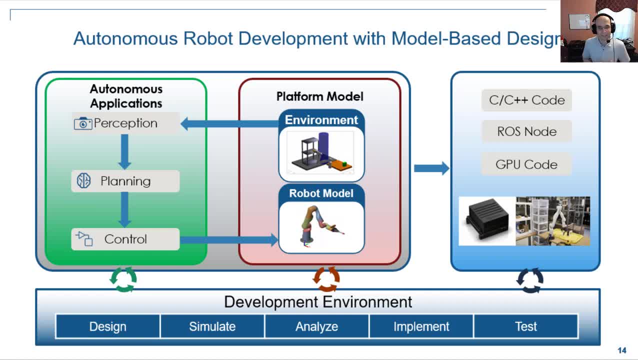 you want this to run on the real robot, right? It has to run in the factory, not in your lab or in your simulation system. So it will be ideal if we can reuse all these pieces that we are building continuously and design, simulate, analyze, implement. 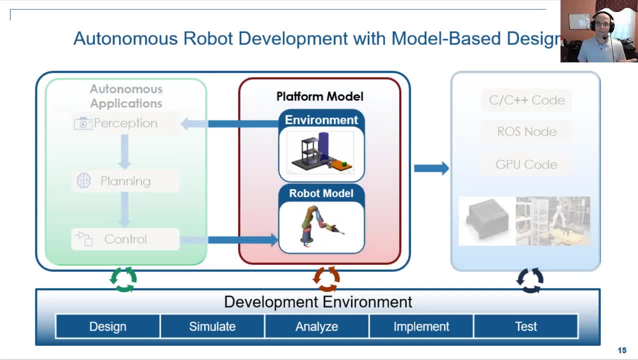 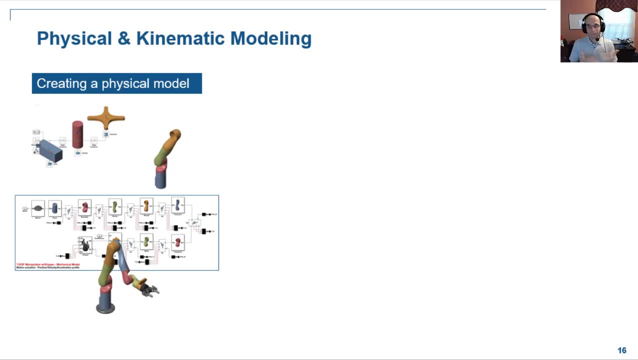 and test our system. This is the promise of model based design And, as the name says, it starts with the robot model, And this is really a crucial step for everything else that follows. So robot manipulators consist of multiple components, right. 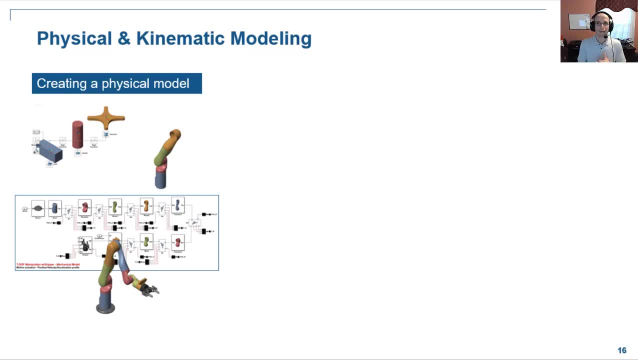 Including mechanical actuators, electrical parts and, you know, potentially also hydraulic parts, depending on how your manipulator was structured. So how do you build a model like that? You can, you can certainly build it from the bottle up, from individual components, right? 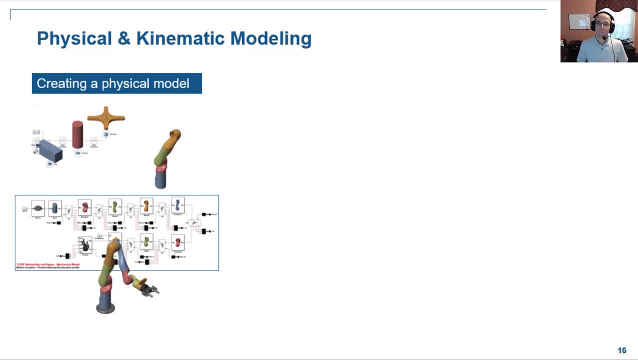 Connecting different links with joints. but more likely than not, a lot of our industrial robot manufacturers have existing CAD models of those robots And you can use those also as kind of your initial truth, if you want, about the sizing and the weight and the inertial properties of that robot. 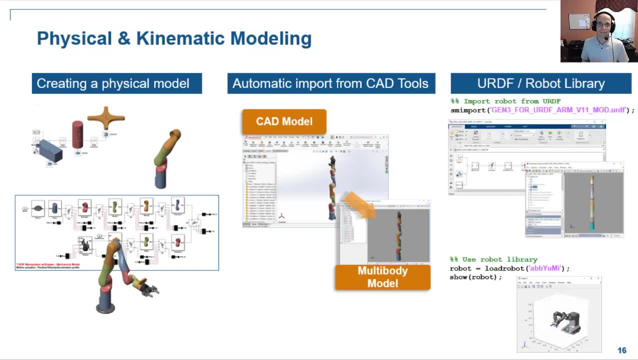 Another popular way to get this model is from the URDF format. If you're not familiar with it, it's. it has been popularized by Ross and Gazebo And nowadays, really most robot manufacturers provide URDF descriptions of their robots. 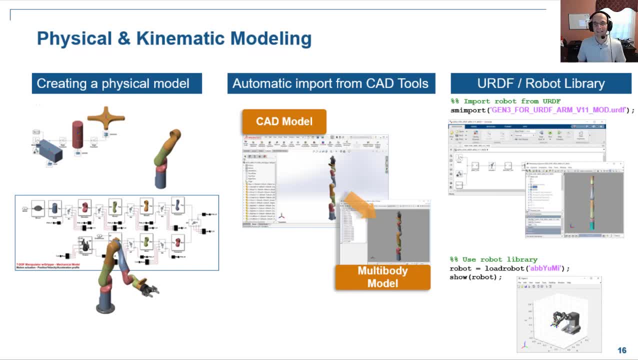 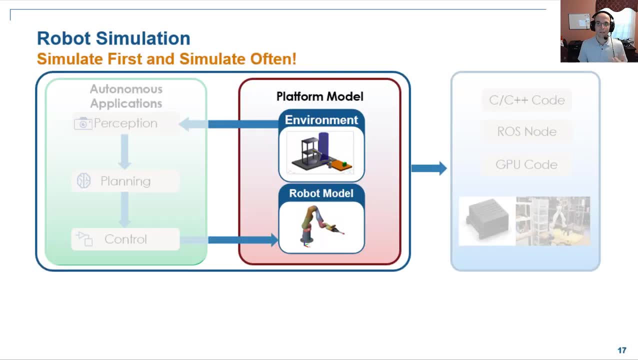 So this is a very handy way to quickly get the full description of a robot into the software of your choice. So conducting experiments with real hardware is expensive and time-consuming, as you probably know, And sometimes it might even be dangerous when you are first trying to tune your controllers. 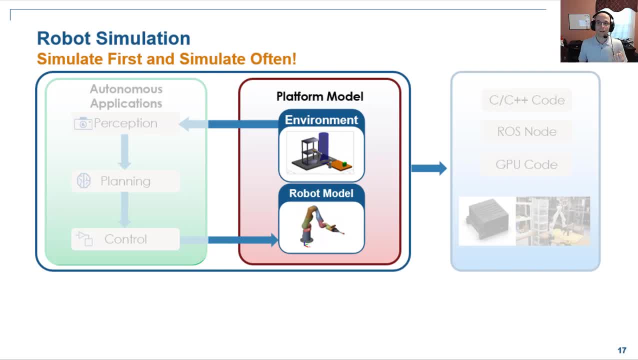 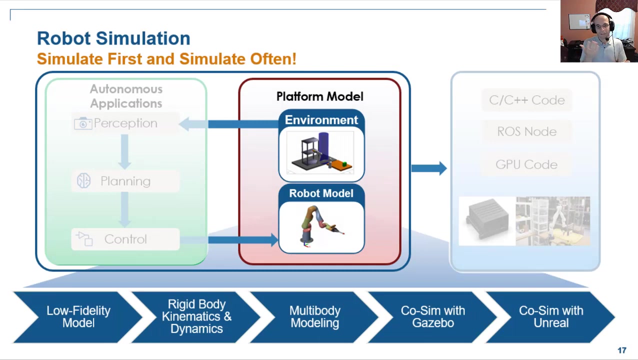 So simulation is really a powerful tool for analyzing, optimizing your algorithms and really taking a robot model into account, right Building the algorithms to deal with the complexities of your model. So for many workflows, like testing and debugging your system, the physical system is replaced. 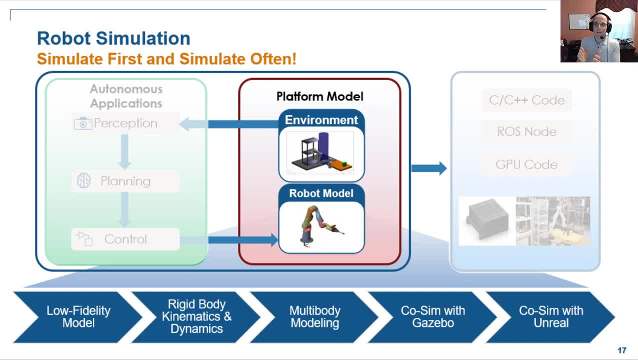 with a simulation right And the simulation could really happen at many levels, from a fairly simplistic, low fidelity representation to a high fidelity, complex simulation. It turns out from many, many companies we talk to this is easier said than done. Like, how do you do this? 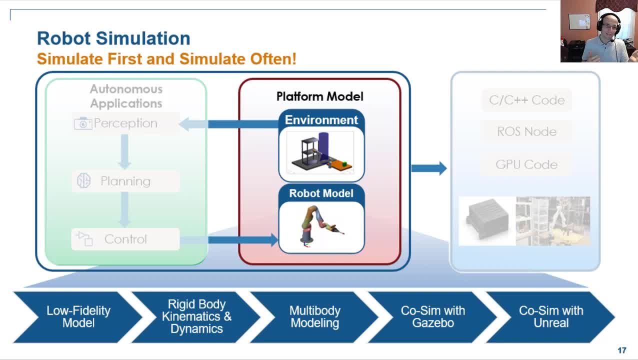 How do you go from a simple representation to a more complex representation? And one thing you need to keep in mind: in large companies you have tens or hundreds of engineers working on the same problem. They don't all need the same simulation complexity. For example, a control engineer designing a torque controller. 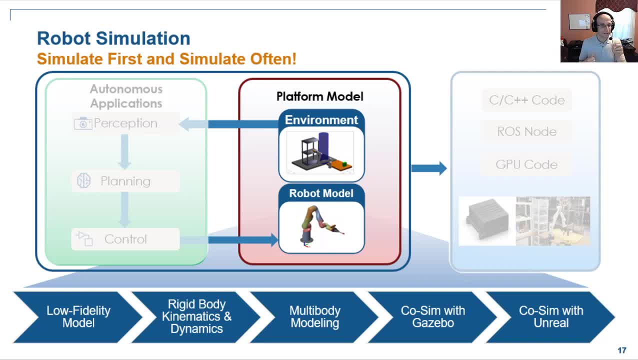 needs the highest possible simulation fidelity to account for all dynamics, all dynamics of the robot. when they tune their controller For an engineer that works on path planning for painting, let's say their input to the simulation is simple waypoints. They assume that that simulator will figure out how. 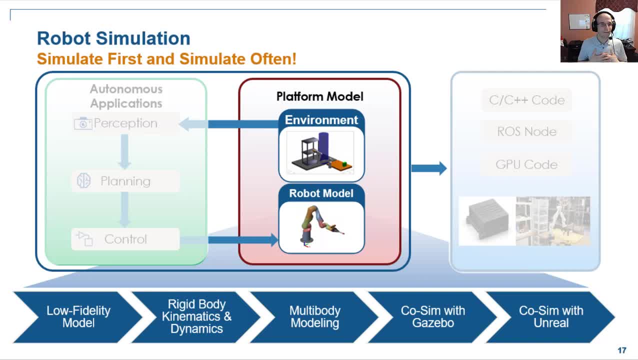 to interpolate trajectories, So their simulation model can be much simpler. So let's discuss how this range of different simulation fidelities could be used. All right, So let's look at some other examples. Were there any models that we can use for göstering? 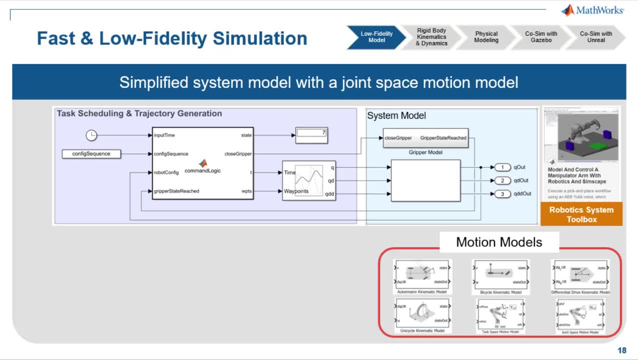 those bow lines. Share that with us. So let's have a look at another model, and I'll give you three examples of models that can be used in a different way. These models will be extremely useful if you're going to develop plan altitude. 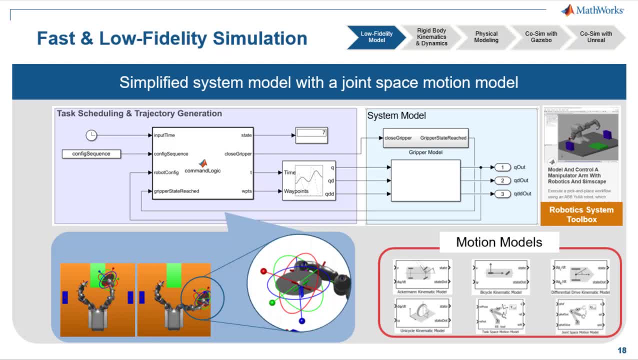 and these models will give you a very clear idea of the plan height, and these models could be supported through model-based design. All right, Let's give some concrete examples. Right At the early stage of application development, you may focus on the task scheduling of the robot. 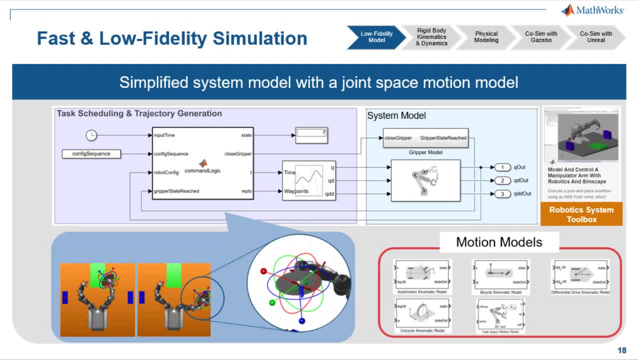 Right your system as a simplified motion model, which is really just a fancy way of saying that this includes both a basic plant and joint controllers. So when you start out, you might not even want to deal with the control aspect, but you simply assume that this is a robot that can be controlled. 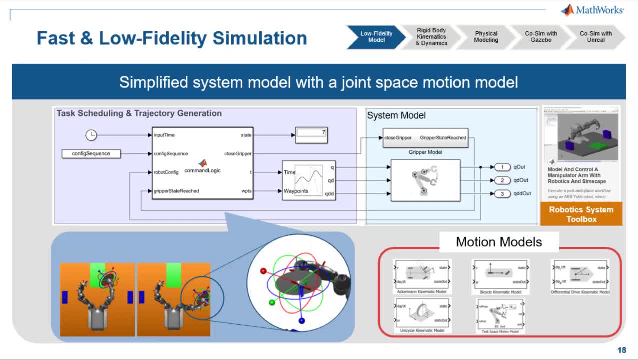 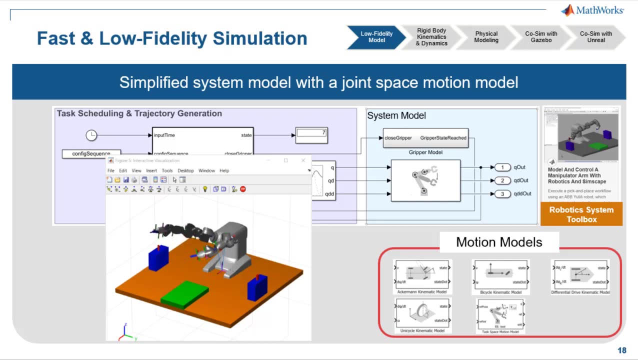 via high level commands. Note that we also don't really pay attention to any grasping at this stage, but this already gets you started to a good degree and you can run simple simulations like how this Yumi robot is. you know, picking up an object and then dropping it in a different spot. 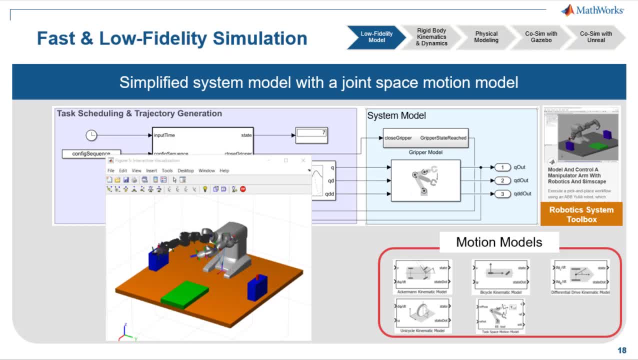 Again, we're not really modeling any grasping here, but you can very easily test basic trajectories with this. So later on you probably want to upgrade this model to something different. You could change it to something else like this, but it's pretty easy. 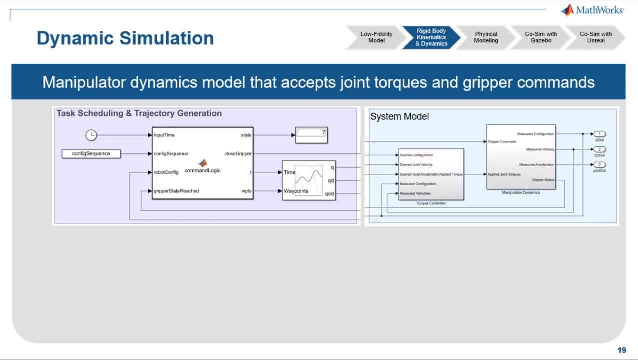 So later on, you probably want to upgrade this model to something more complex, something that's closer to what your real robot, how your real robot behaves. So after this kind of task scheduling has been designed and verified, you probably want to model the controller for your robot. Again, a more complex manipulator dynamics model is needed. 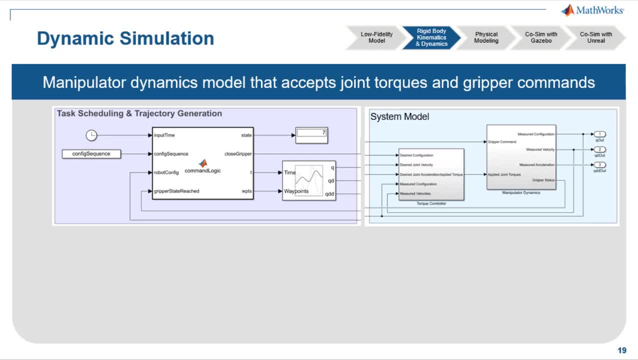 that takes joint torques and gripper commands and you probably need a torque controller for this robot. The power of model-based design is that the rest of the system model stays the same, So you can run the same verification test as before and verify that your arm behaves correctly. 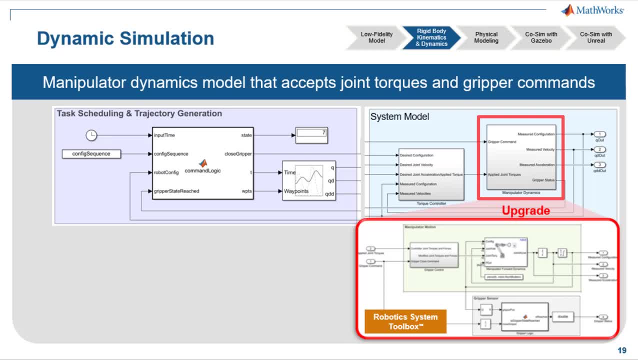 Again, here's just one example: in the tools that we built here at MaFox that would simply allow you to iteratively replace your robot model with higher fidelity components. And again, you probably want to verify: run the same automated tests, for how would the robot? 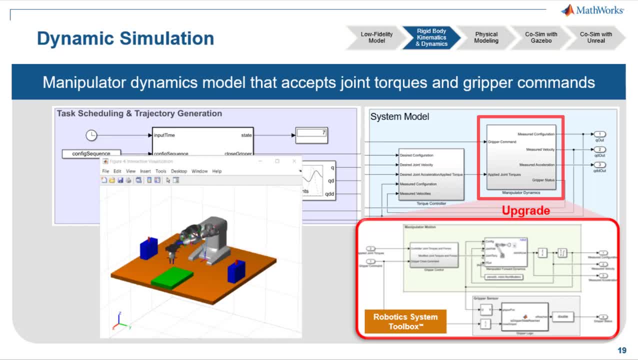 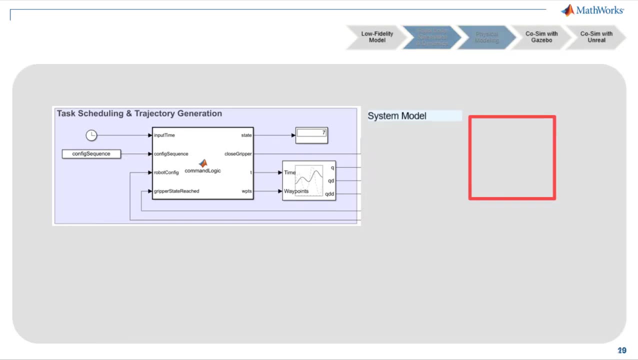 behave when it picks up an object and then drops it off in a different location. But again now likely, you will model more dynamics of the robot and you can tune your actual torque controllers for each of the joints. Now we can add an even higher fidelity model. 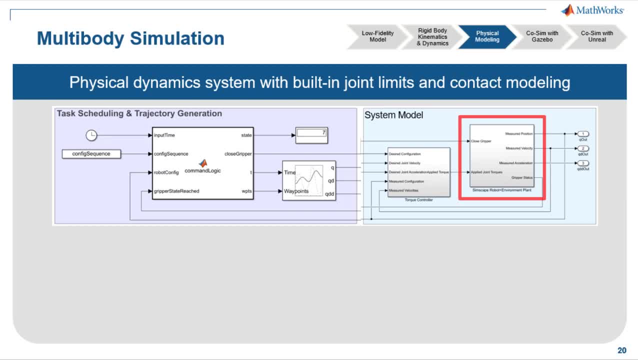 Again defining each of the mechanical parts of the robot, if you so choose, And you might also add other modeling details, Think of the electrical system or the hydraulic system. The main difference from the previous model here is the plant. The plant model now. 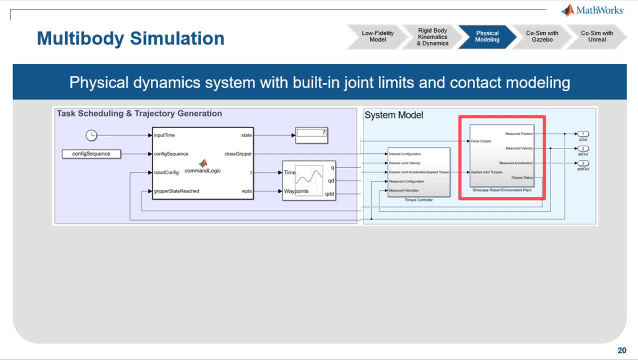 incorporates the full dynamics of that robot with built-in join limits and contact modeling, And this simulation accuracy can be achieved with many tools. From MaFox perspective, we have a range of software tools for physical modeling And it helps you to really get accurate simulations. 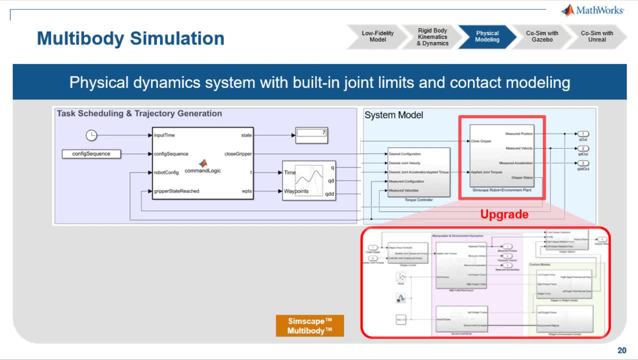 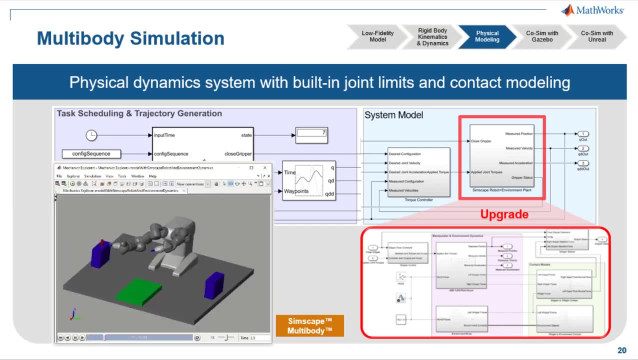 but it comes at a cost of simulation speed, Whereas in the beginning you could quickly iterate over different task schedules for your robot and quickly change basic behaviors of the robot and simulate that as often as you want. This more complex simulation takes time And that's why you want to follow this process of iterative design So that once you 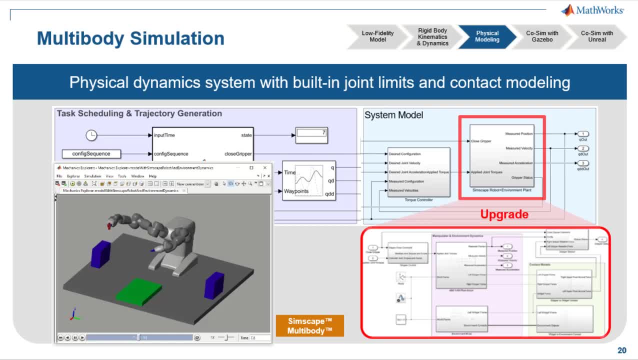 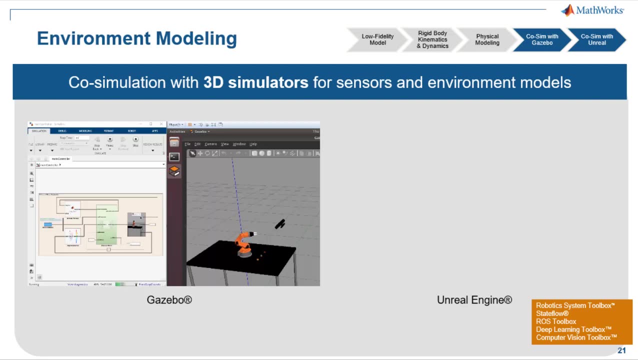 get to this high fidelity simulation. there are really not that many parameters to tweak in the algorithms you're working on right, Because, again, simulations are more expensive in a higher fidelity environment. So one thing that is still missing from the simulation is a proper representation. 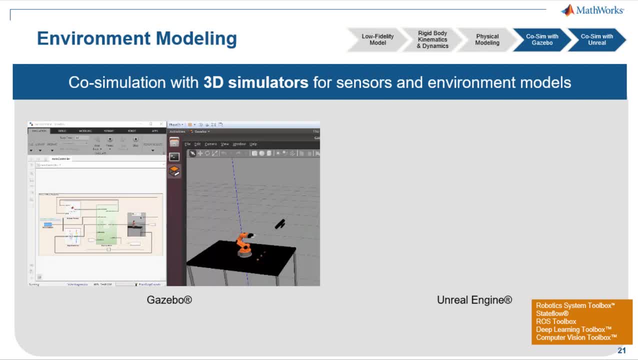 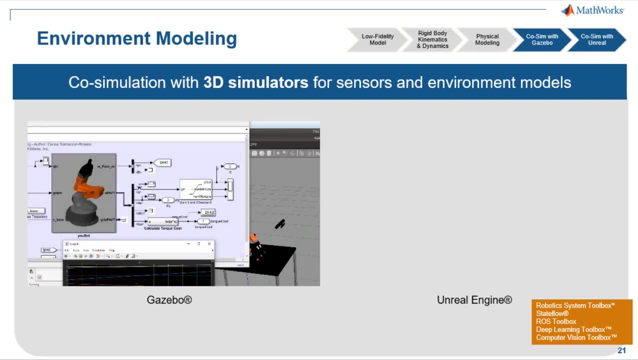 of the environment and the simulated sensor readings from the environment, And this is usually the time when you need a more full-fledged 3D simulator. In this case, here I'm showing Gazebo, which is a popular simulator for robotics And 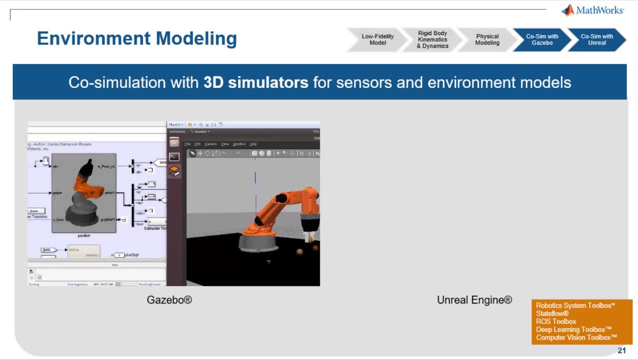 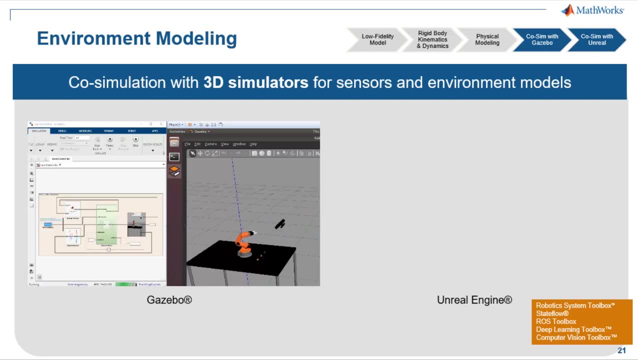 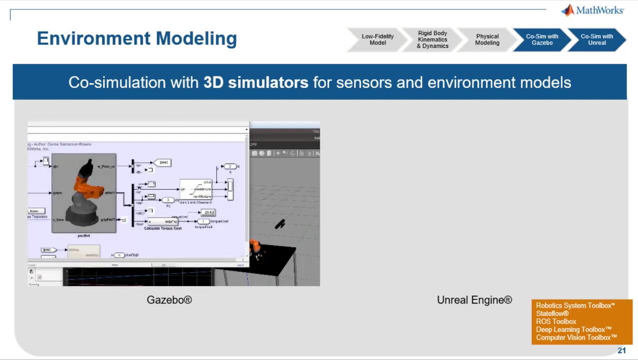 again, you might want to use Gazebo, Because it has a richer set of tools for specifying the environment around the robot And because it has a set of built-in sensors that can be simulated, for example, cameras, depth cameras, lighters, and so on. Again, the ideal place for model-based design is 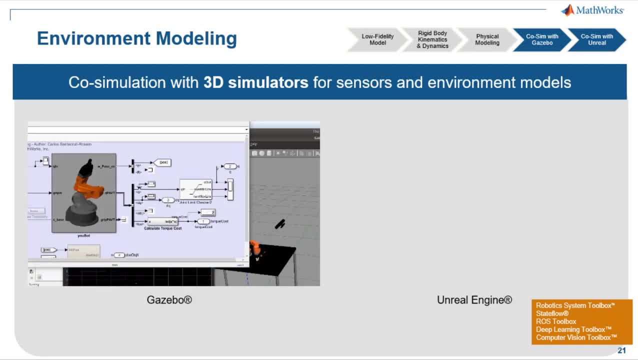 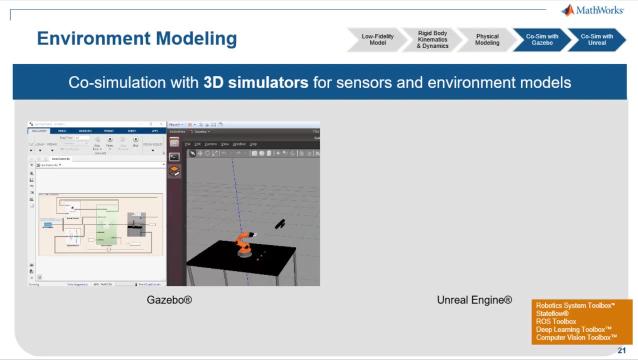 if you can reuse all the model pieces you already developed but simply replace the plant and sensor models with data coming from Gazebo Again. that's, you know, from our company's perspective. that's where we help lots of companies that want to leverage the latest. 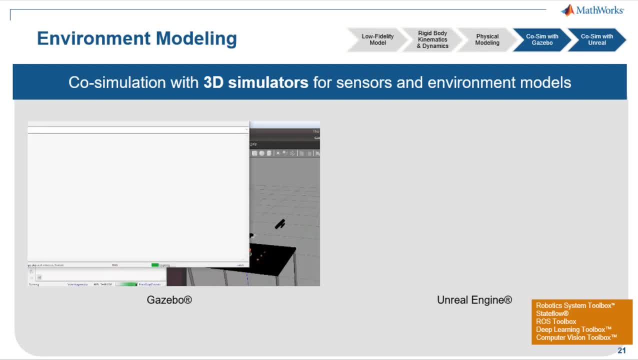 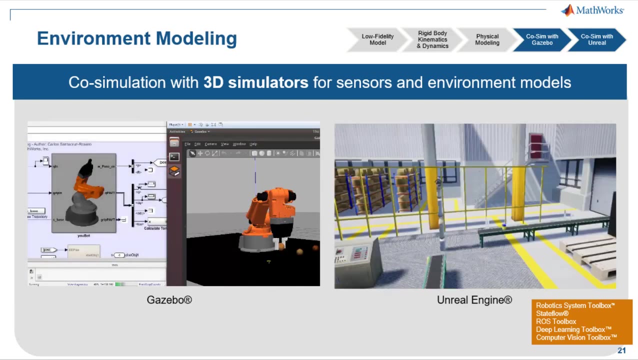 robotics simulation tools, but also want to leverage all the years and decades of work they put into their MATLAB or Simulink models for their controllers. But Gazebo: one drawback it has is the graphics are a bit antiquated, So actually a lot of. 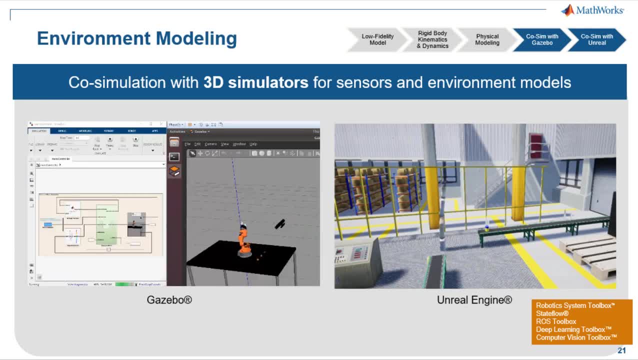 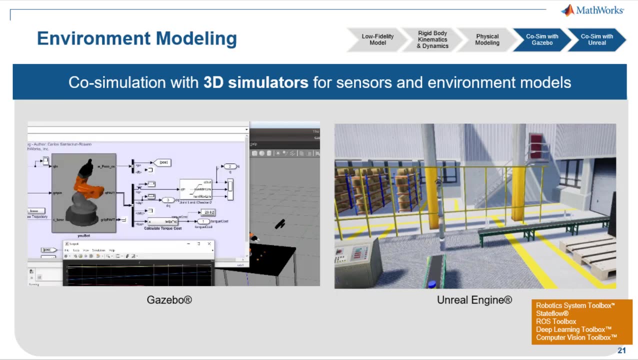 companies would use other tools for simulating more photorealistic scenes. This is great for things like AI and deep learning, where you need photorealistic camera images for training your network And again you want that transition to be as smooth as possible between the different tools you're using, And a lot of customers don't want to deal. 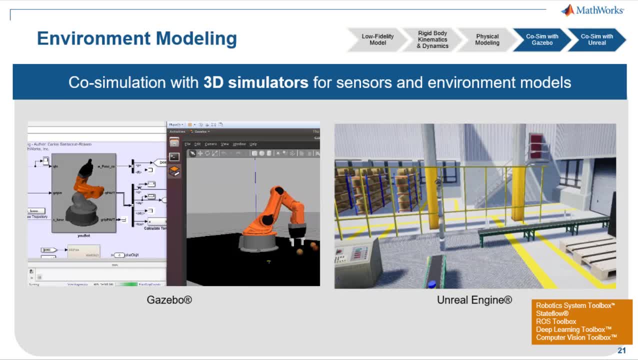 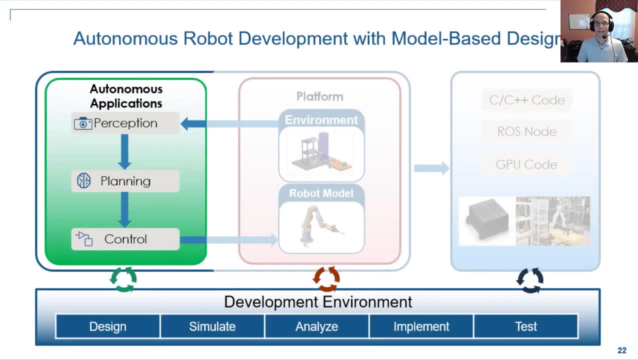 with the hassle of switching to a new simulator and then having to change all the tools or code they've already written. All right, moving on to the next pillar, right Adding autonomous algorithms for perception, planning, control. Again, we have a robot model. now we have 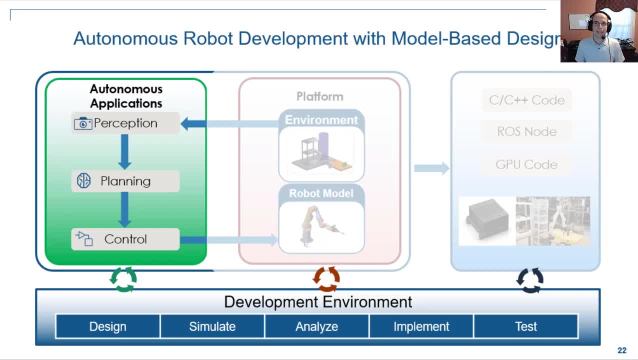 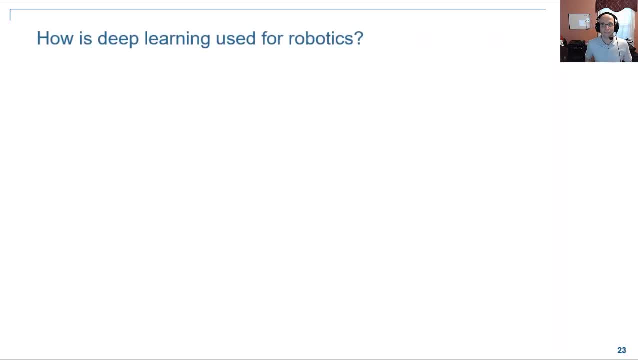 simulated sensors. How do you add algorithms for autonomy? And before we jump into a perception example, let's look how deep learning can be applied on a robot. Again, there are lots of ways that deep learning is really transforming robotics and also starting to have an impact on 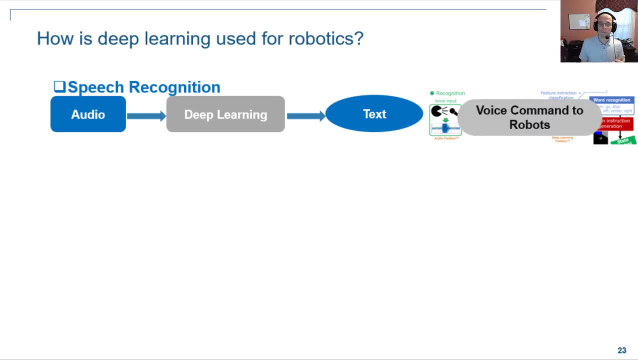 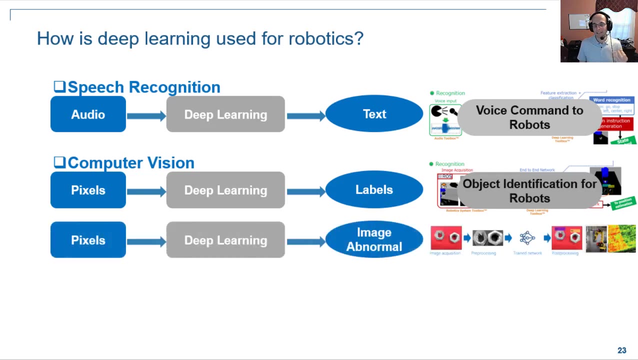 industrial robotics. One is for speech recognition for robots. The more traditional deep learning application is to detect objects- and this is great for pick and place applications- and also detect abnormality in parts manufacturing. LIDARs are also starting to have an impact, or depth cameras, because they provide a more spatial 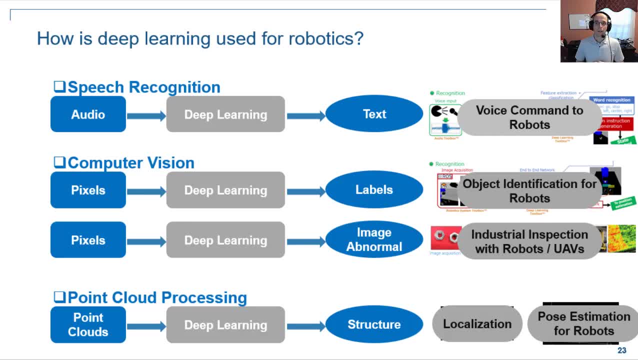 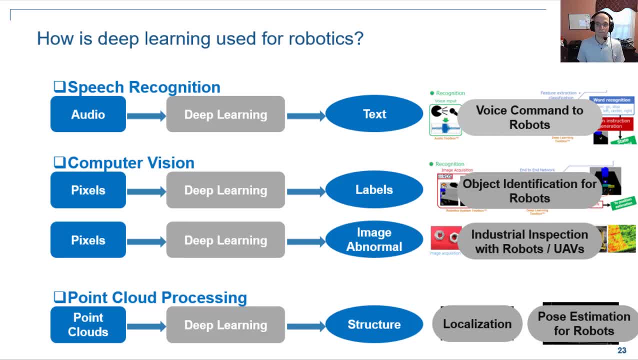 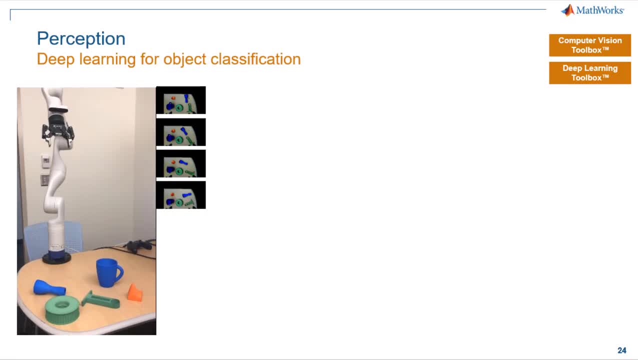 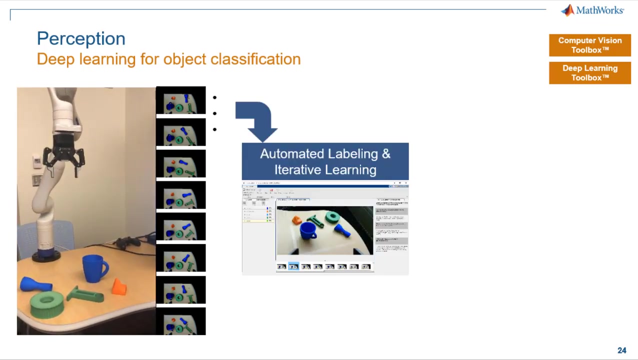 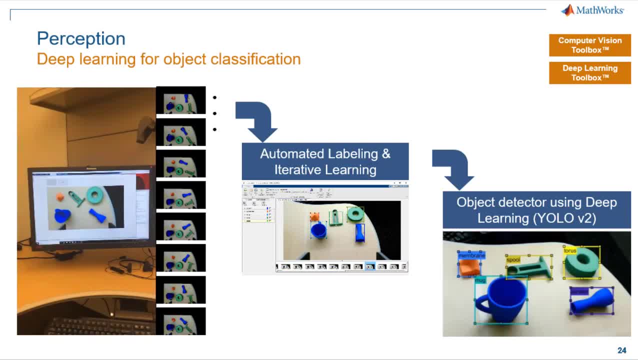 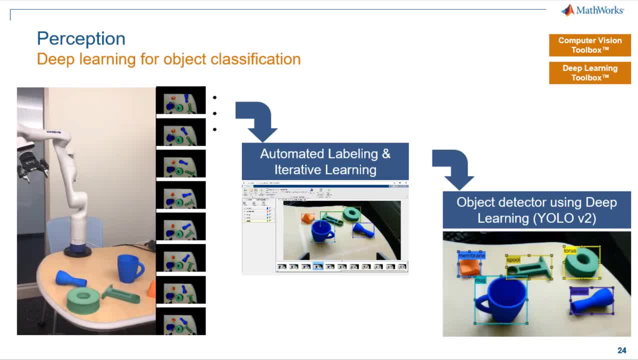 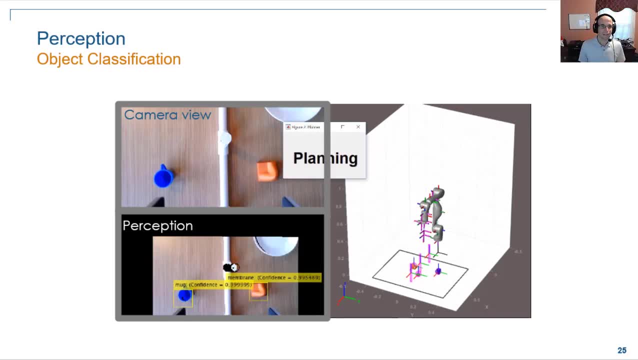 In this case. here it's using the fairly common YOLO architecture. So here you can see an example just from the robot's perspective and how deep learning based object detection is used in conjunction with path planning for real robot. So one thing that I should note here is 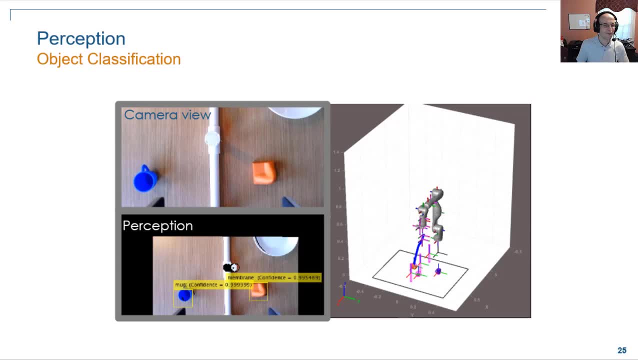 so deep learning has been around for a while now and we all know its benefits. Interestingly enough, most of our industrial robotics customers are interested in deep learning, but really only for systems or parts of the systems that don't impact the safety. So, for example, advanced bin picking systems. 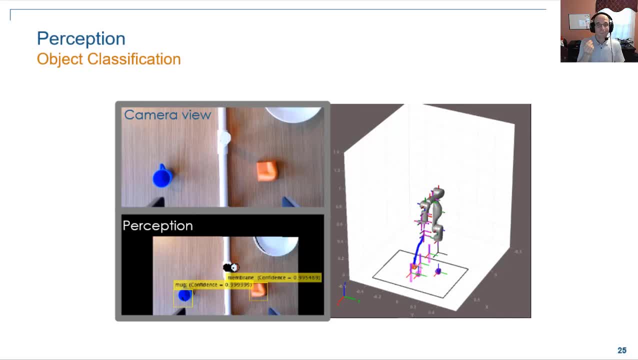 leverage deep learning for object recognition, But you don't really want to have a deep learning network control the robot motion, And the main concern there from the companies we talked to is that functional safety and the ability to certify systems are major considerations And deep learning is a challenge to fit within the certification framework. 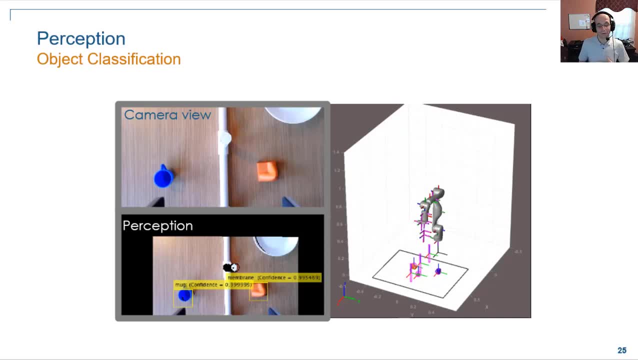 This is not new. Automated driving is dealing with this right now. That really a lot of the tried and true techniques for certifying safety-critical systems, Um are not easily applied to systems that employ deep learning and artificial intelligence. Again. industrial robotics companies are even more conservative. 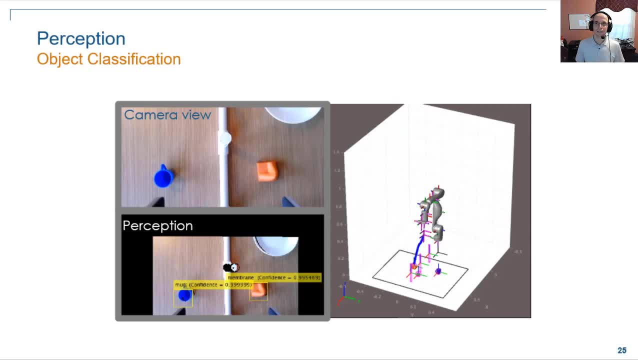 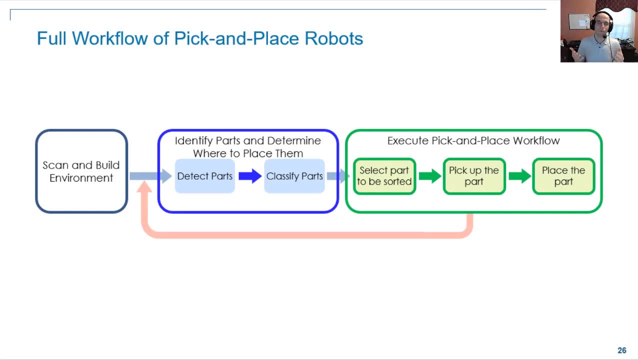 But again, deep learning is starting to have an impact on perception related tasks. So now let's look at a higher level workflow for pick and place. So here's a basic flow chart of kind of the pieces of each pick and place application: Um, from uh sensing the environment, identifying parts and then executing a pick and place workflow. 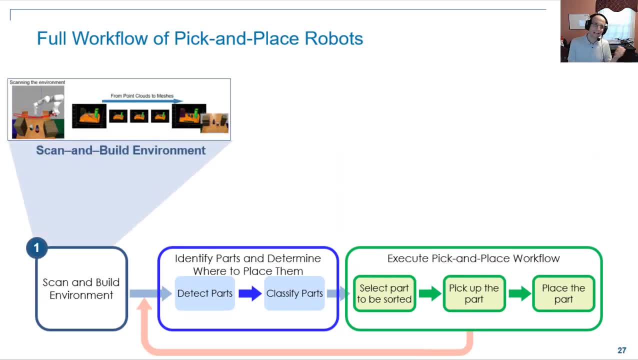 And you know. in traditional pick and place environments, again, everything is known beforehand. You know where parts are, You pick them up. you do it repeatedly. For co-bots and smaller factory environments you likely have to use sensing to find objects. 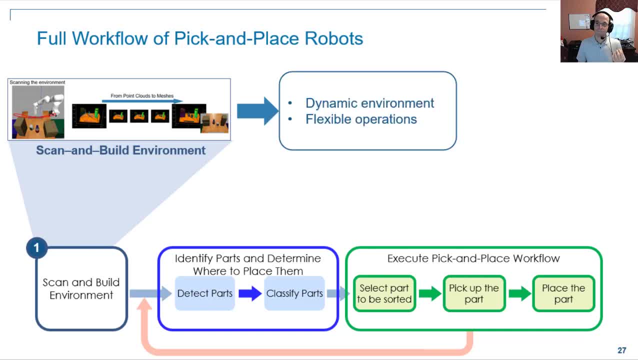 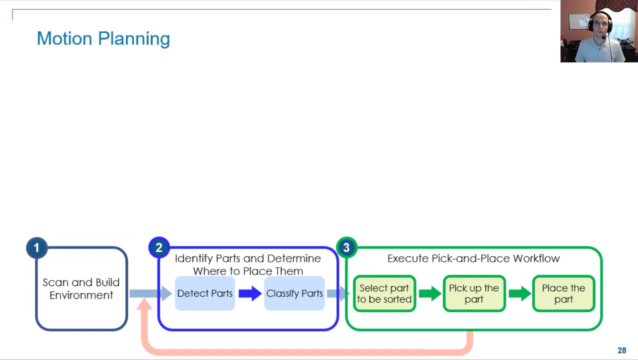 And you know I already discussed um. I showed you an example of how this detection and training might happen through deep learning. So one thing that we're interested in now is how do you execute this pick and place workflow. How do you deal with motion planning, control and hardware connectivity? 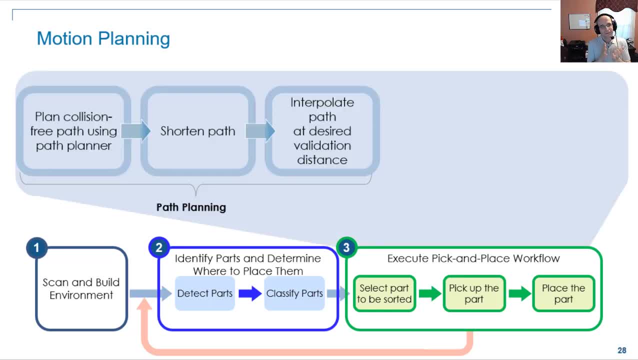 So let's talk about motion planning and there are really two parts of it and to most of you here as roboticists, these might be obvious steps within the motion planning workflow. To many of our industrial robotics customers, this is really fairly new. They've been dealing with manufacturing software tools, so software tools from the manufacturers. 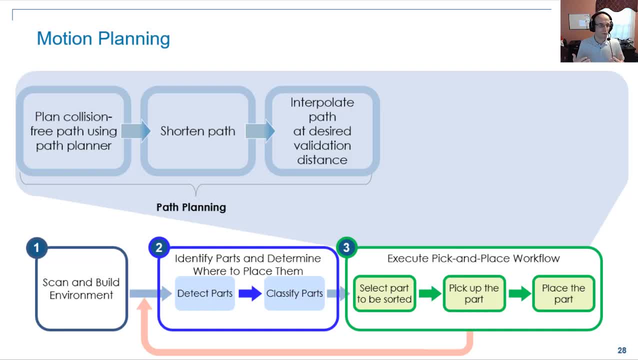 that essentially have done this motion planning for them, and all waypoints were pre-specified and the motion plan was automatically generated. Now for more autonomous systems, some of these tasks have to be solved on the robot and have to be customized, So it's actually interesting to see how they approach this problem. 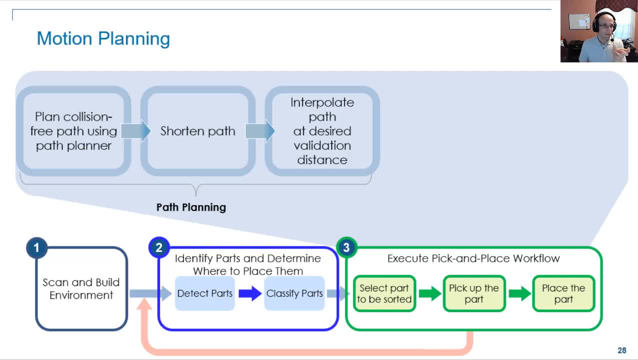 And typically motion planning is subdivided into two parts. right One is the path planning, meaning finding a collision-free path that your robots can go through. It's typically at the waypoint level and in the end you want to interpolate a trajectory. 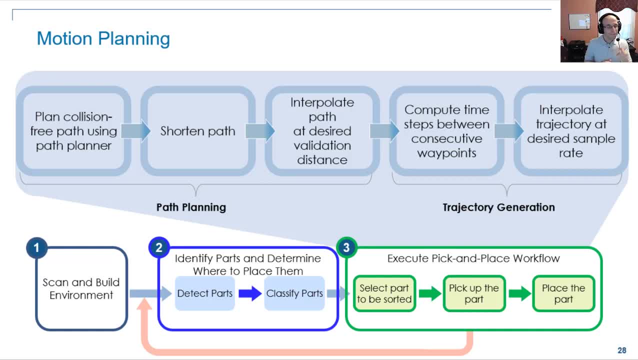 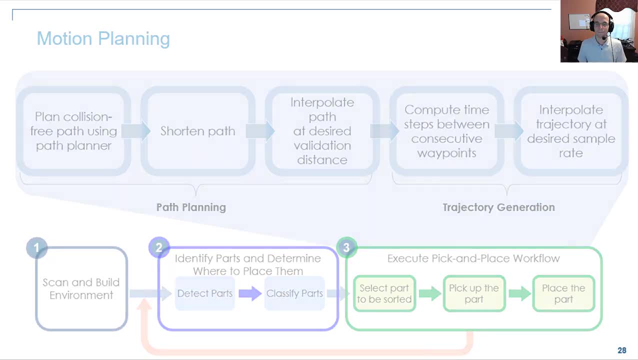 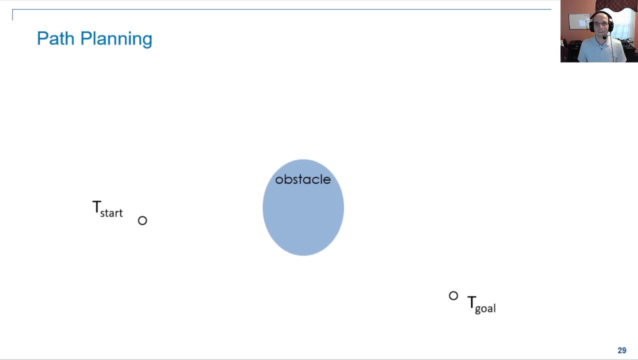 that your robot can actually follow and that minimizes some kind of criteria. For example, a popular one is minimum jog. But let's start with path planning, right? I mean just to get everybody on the same page. the problem of path planning is really starting. 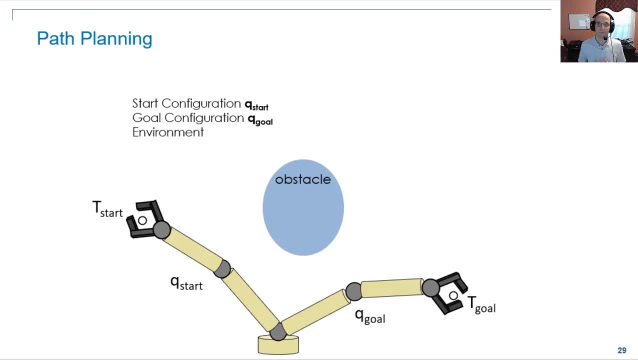 with an initial pose and a final pose and some kind of environment representation And then, as a first step, most path planners right relate these poses to actual start and goal configurations of the robots, typically using inverse kinematics, And then the planner aims to connect these configurations. 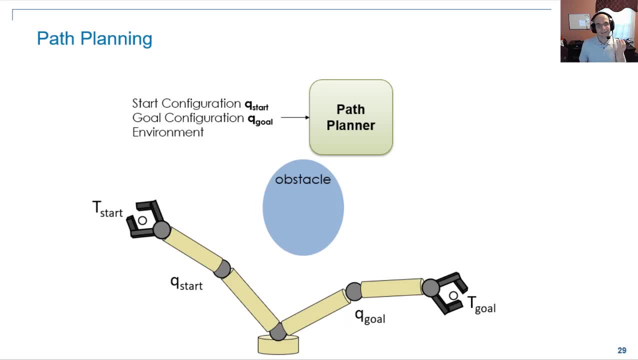 And what makes the problem more interesting is that there are certain constraints on the planner. These constraints might be obstacles, static or dynamic obstacles, Or things like joint limits, And then the path planner will find a collision-free joint trajectory that gets the robot from. 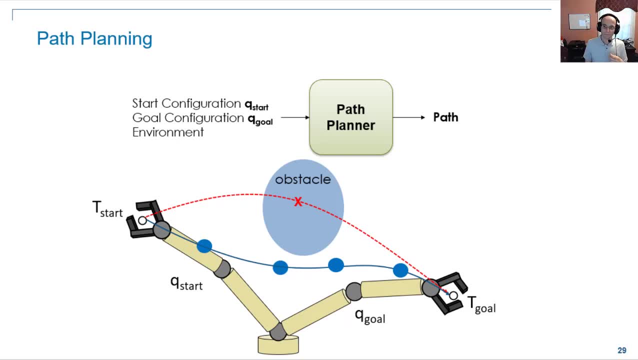 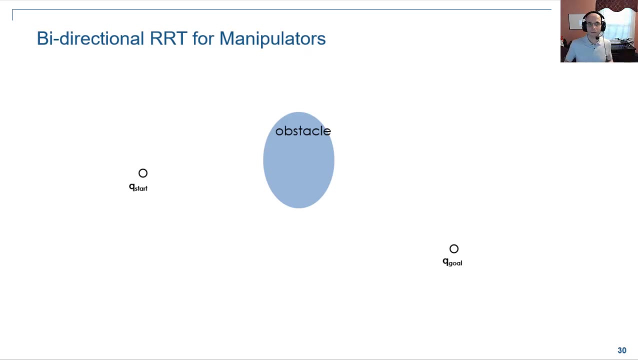 the starting position to the end position And depending on the characteristics of the application right. you can either solve this through optimization-based approaches or sampling-based planners. These are the most popular ones in industrial robotics. One sampling-based planner that's especially popular is the bidirectional RT. 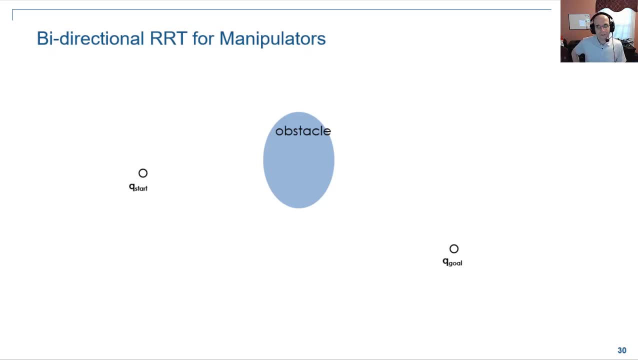 And I'd like to explain this planner a little bit. So bidirectional RT planner creates two trees And one starts from the start configuration and one starts from the goal configuration And these trees grow outward and the planner seeks to connect them, to find a path that 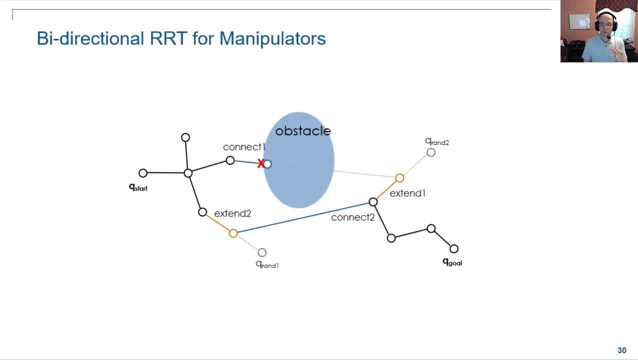 goes from start to goal And the planner uses several heuristics to reduce planning times. So one thing you see right away is it's a sampling-based planner, So the waypoints you get are really dependent on how finely the planar samples the space. 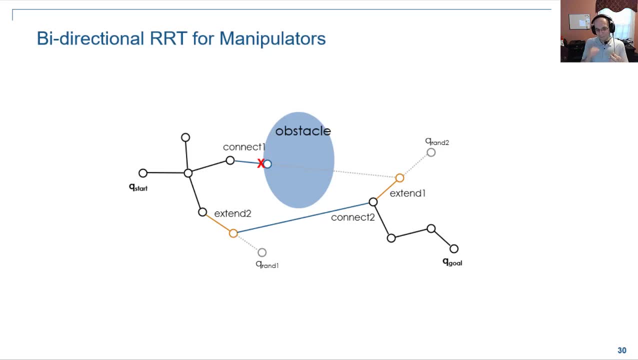 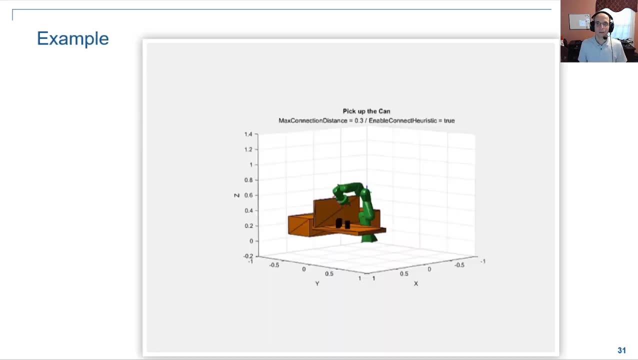 And the resulting trajectory- if you just connect the waypoints- is likely not a trajectory that you want your robot to follow. It's not going to be very smooth. So here I'm showing just one example of how this planar would solve a pick-and-place problem. 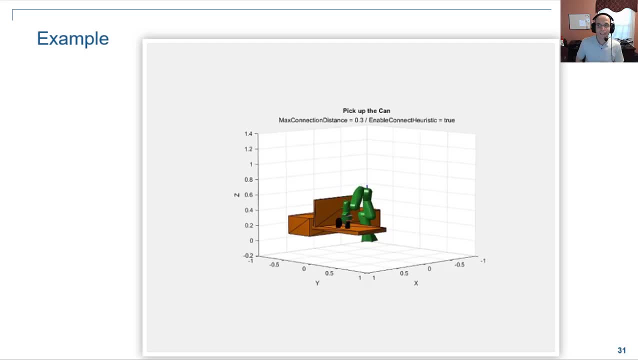 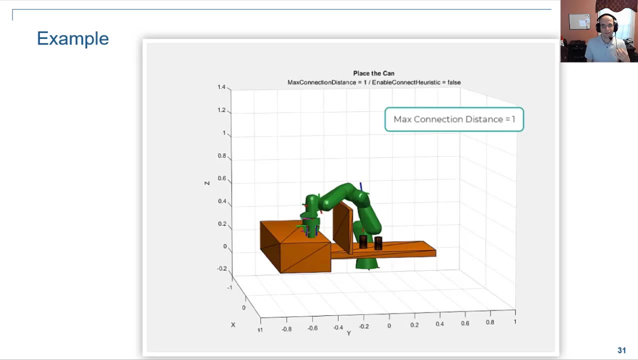 And where the robot first picks up the items on the right and then moves it over the obstacle to the table on the left. And the only thing this example is showing is that, depending on your problem description and the type of obstacles you have, the type of robot you have. 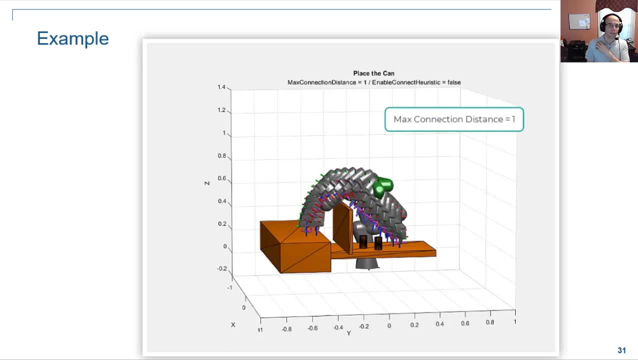 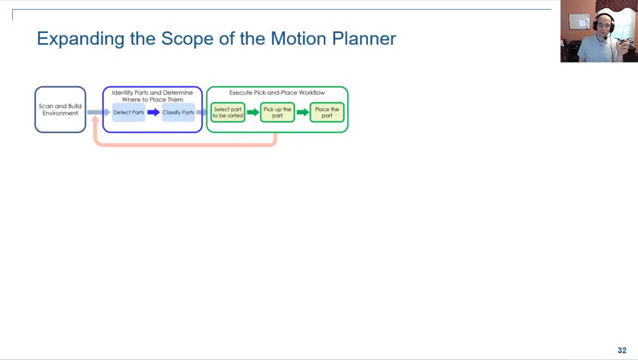 you probably have to tune that planar to find the best parameters for your particular application. So up until now we've been assuming that you can place, You can plan- configuration to configuration. but many pick-and-place applications are more broad than that, right. 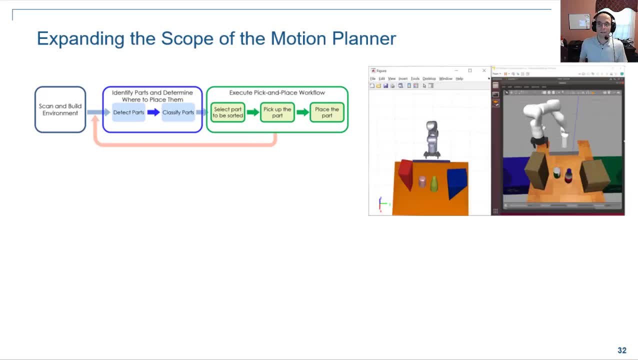 You don't just go from one spot to the next, but you also have to dynamically scan your environment and detect obstacles, And that's really when your planning starts. So it might be a dynamic environment, not just a static point-to-point type configuration. 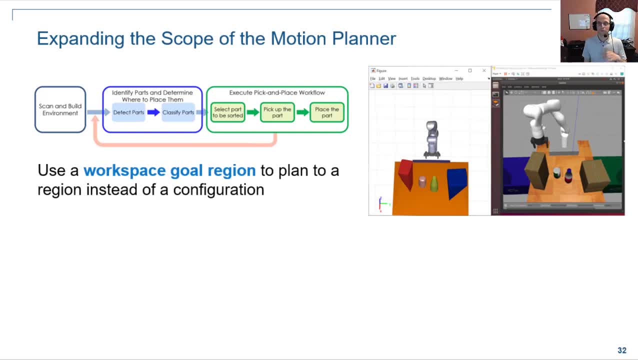 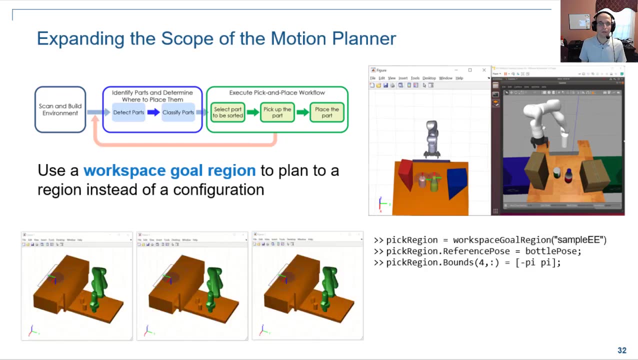 And in applications like this, what might be more ideal is to planar. You plan to region rather than a specific configuration, And the workspace goal region is a popular approach there, And here are just a couple of videos that show how you can not just define where your robot should go exactly. 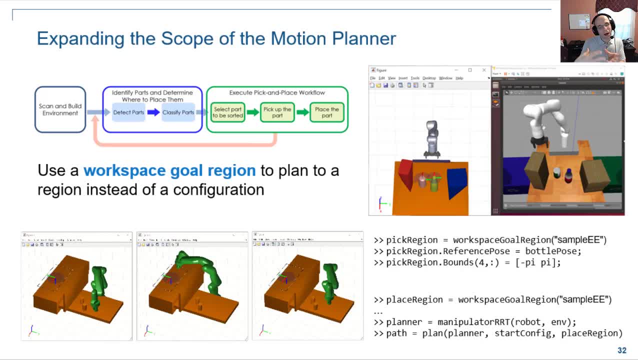 but define different boundaries around the goal. Think of them as there might be a region you can go into, Or you might have a certain tolerance around your end effect or pose at the goal location. So all that really helps in ensuring that you can execute the robot motion while the environment might be changing right. 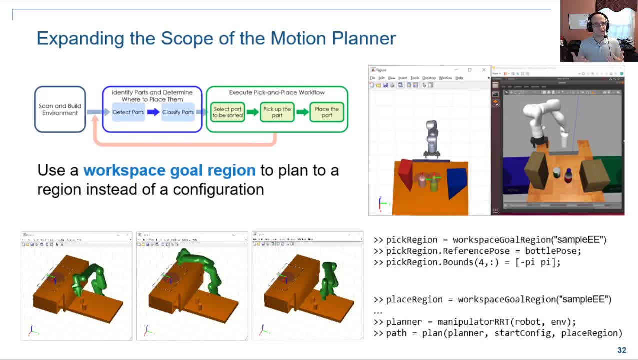 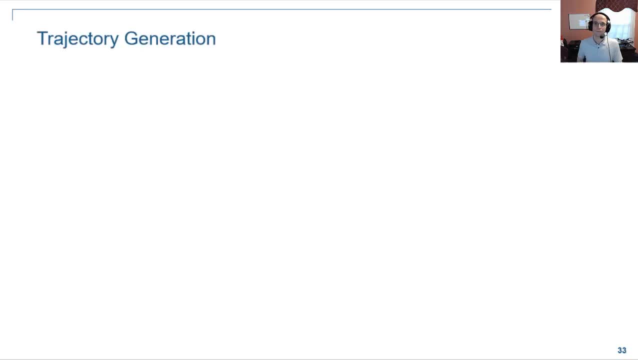 So, rather than sticking with a fixed plan, something like a workspace goal region allows you to react more dynamically to changes. So, to review, we started with a set of input configurations to you know, pick and place and then use the path planar to get a path. 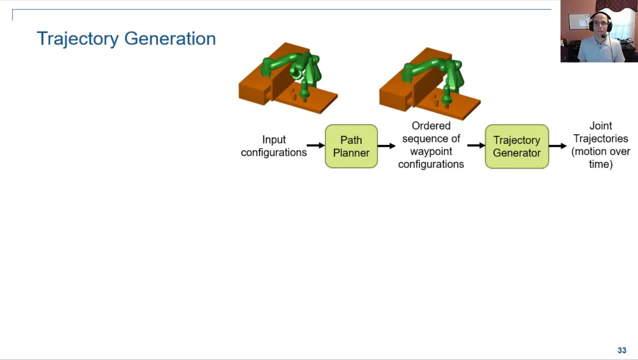 which is kind of an ordered set of waypoints. But when we actually pass this into the motion controller, that's not enough right? You need some kind of time association, like when is the robot supposed to reach these waypoints? And that's really where trajectory generation comes in. 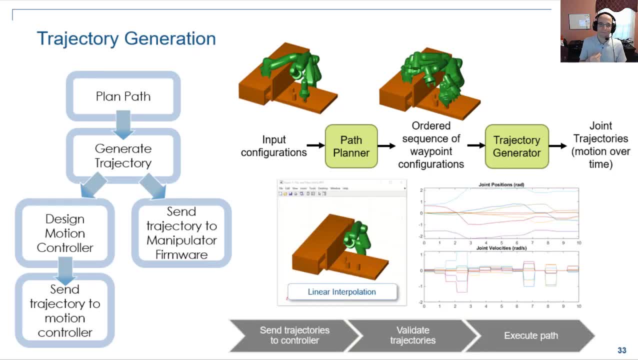 And one intuitive way of doing this would be simply to interpolate the positions in joint space. But the problem with that is that obviously that leads to non-smooth trajectories, which is really not desirable because it leads to extensive wear and tear on the manipulator arm. 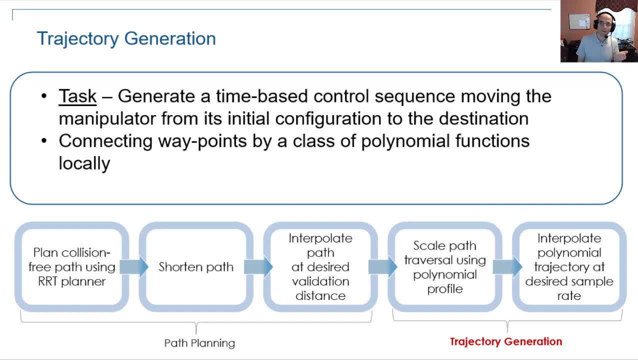 So trajectory generation really fulfills this task of mapping the organization. You can say you know it's a relational system, right? So as the commands are, what I think you're doing should actually be removed from the COBold configuration. andhun estran ansun. 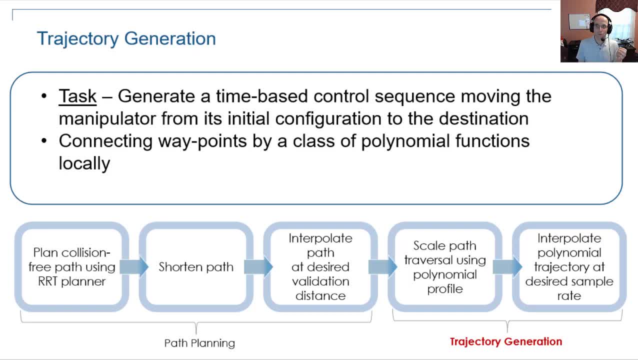 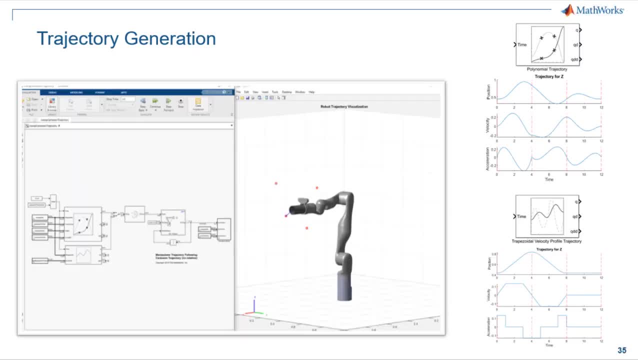 but I think even more to say to practice the trajectory group in order to be able to determine which Jahre rods are continuing. In that sense, is the path planar? myView button is basically going to Triangle taken. you know just a histogram of what kind of traps that happen. if you wanna give control to a unlikely task, to do a little bit of an initial sketch. 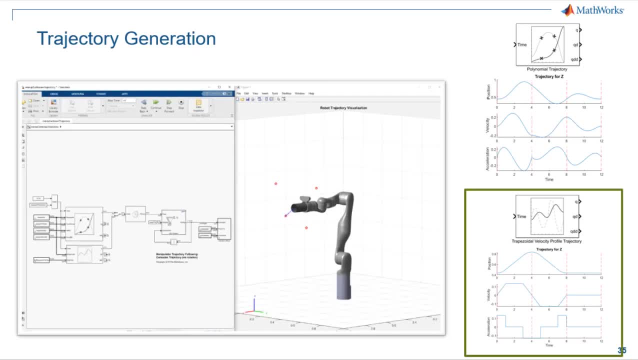 So I think things could do their work very well, right where the end effector is. Trapezoidal velocity trajectories, for example, are using a piecewise trajectory of constant acceleration, zero acceleration and then constant deceleration, And this leads to this, you know. 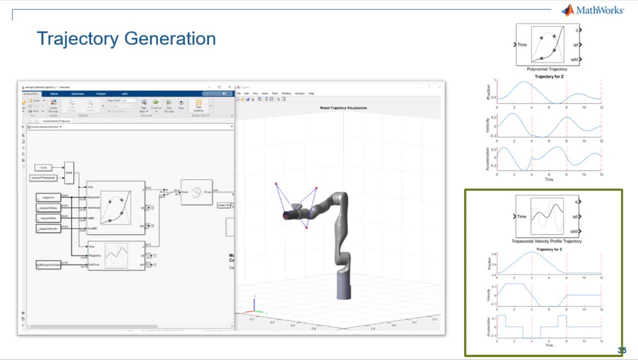 well-known trapezoidal velocity profile. It's relatively easy to implement And but it gets the job done And really most traditional industrial robots used trapezoidal velocity profiles. But you can also interpolate between two waypoints using various orders of polynomials. 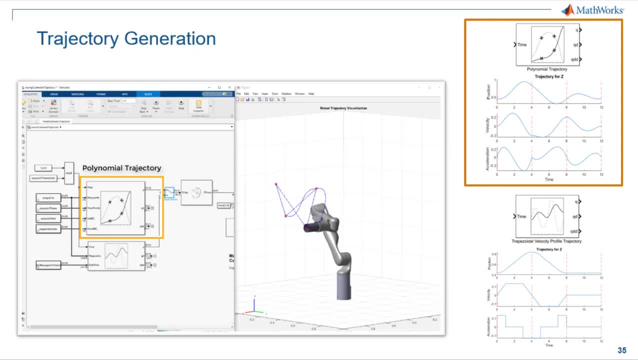 And these polynomial trajectories are particularly useful for continuous motion because the trajectory can pass through the waypoints with non-zero velocities and you can get smooth velocity and acceleration profiles. So the most common polynomials here are typically cubic or quintic polynomials To ensure certain level of smoothness. 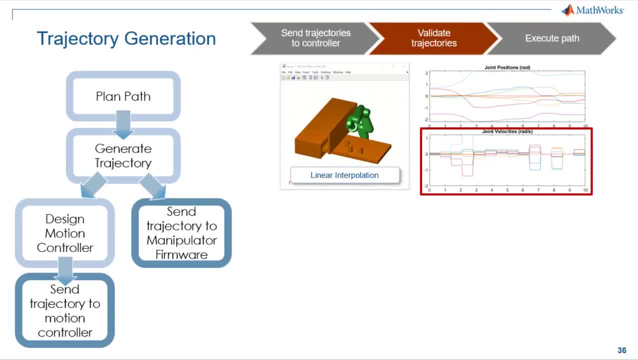 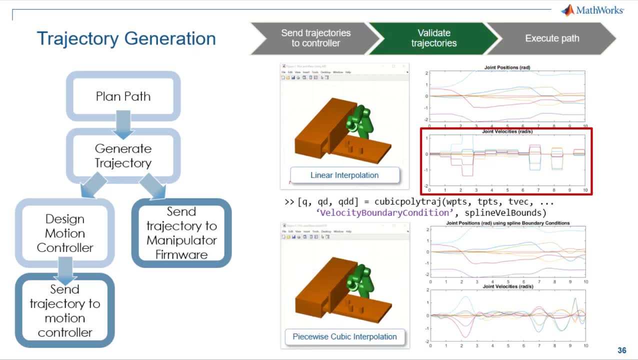 in the derivatives of the joint motions. So again, just to summarize, now you have some kind of trajectory generator, you know. pick one of the many I just mentioned and you can pass that then to your, the firmware of your manipulator. 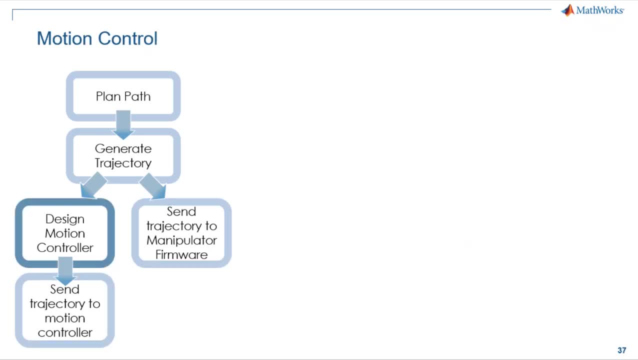 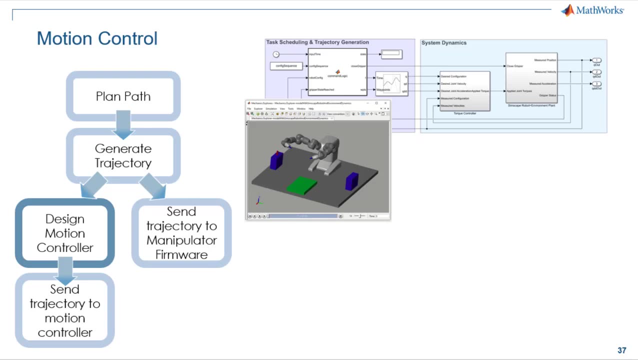 and actually execute this path. So a trajectory provided to the robot can be go directly to the robot, but you can also validate that path, obviously through simulation. Again, going back to the model, this trajectory you can then pass through your modeled. 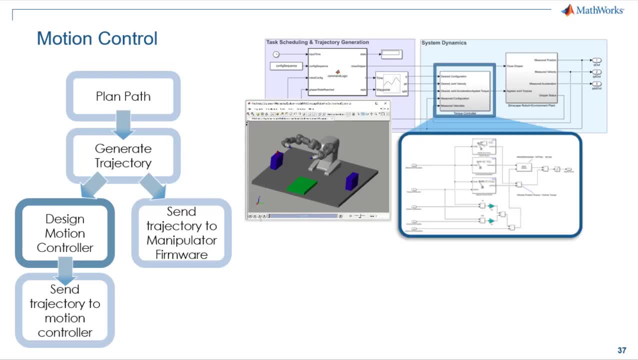 for your robot model and through the controllers that you designed- and you know it's a good way to you know, try out new control schemes and also attuning controllers that you eventually want to use on the on the real robot. You know just a couple of examples of playing. 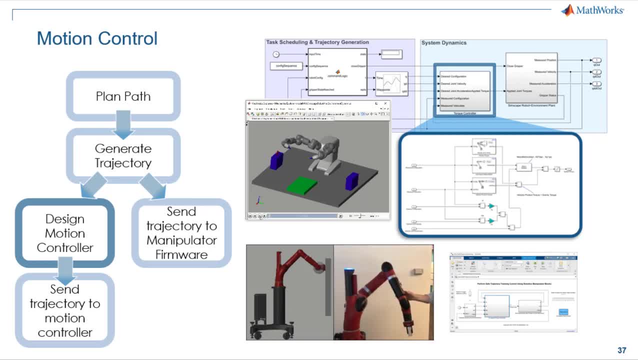 with impedance control. Again, this is a very important way to have the robot react to external stimuli, especially when it comes in contact with objects or humans. So now that I've gone through this stuff, just wanted to show you. you know some. 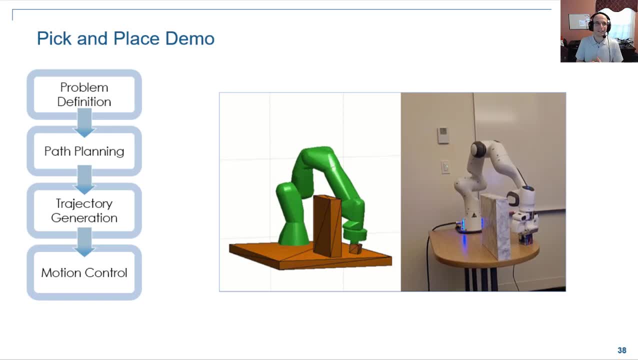 you know maybe the most common points that I've discovered, such as turning the controller back, turn it on and on you model sort of, so to speak. So now that I've kind of walked you through the steps for implementing pick and place from path planning to trajectory generation, to motion control, we can deploy this and run it on a real robot. 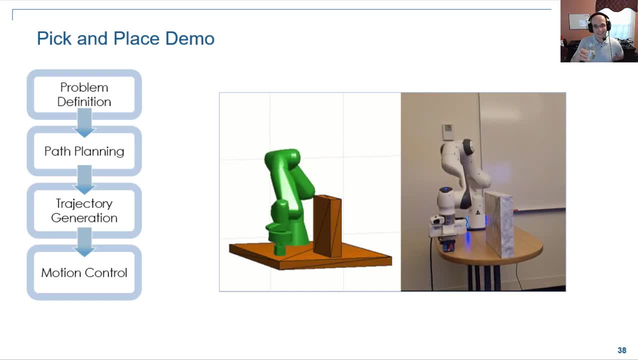 Again, this is just, you know, a little robot that is in our office, But the idea is the same: that ideally, the promise of model-based design is that you can validate your complete algorithm and simulation- see on the left side- and the final deployment is just a click away and that robot will behave exactly the same in the real world. 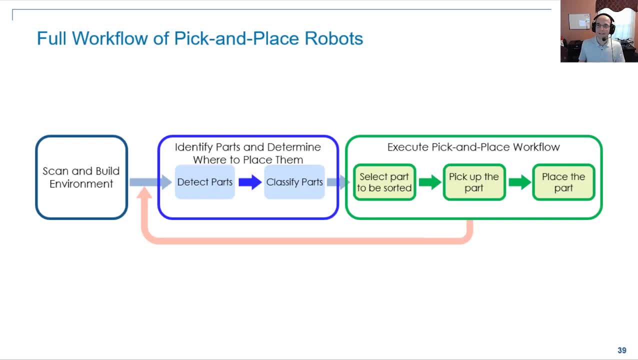 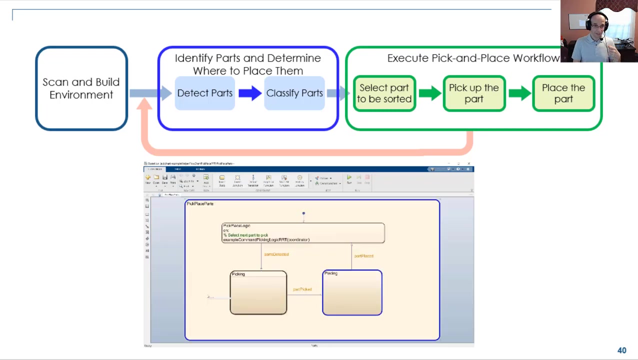 So once you're sure that we can execute this pick and place, we can step back and integrate this workflow Again. in most applications you don't just want to pick a single path, you want to do things repeatedly, 24-7, and as fast as possible. So probably there's some kind of state machine that you also have to implement to run particular tasks repeatedly. 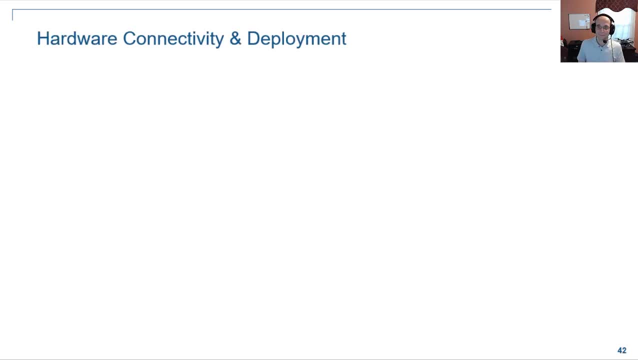 So now let's go to the last step, Last pillar, hardware implementation, And here I'm going to cover a couple of different ways. how you know, we've seen companies connect to hardware, So one option, obviously, is to connect directly to the robot. Many cobot manufacturers have direct interfaces that you can use from MATLAB, from Python, from C++, And those typically give you quite low-level access all the way down to torque control. 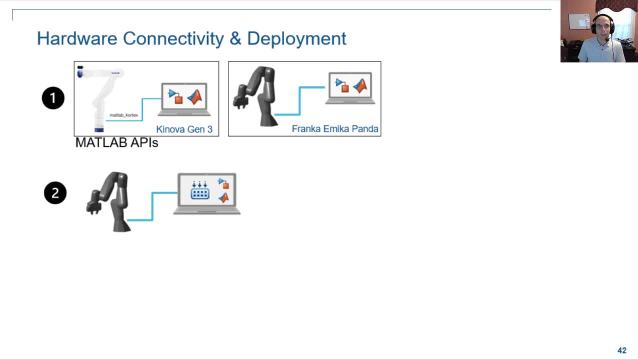 A second option is many of the robots have their own onboard computer And you can run your own control algorithms on those computers, Again through Mathworks tools. we have this mechanism called code generation, which essentially allows you to package up C++ code with your test controller and run it on a range of different hardware tools. A third and popular option that you might have in your head is the Django C++ implementation, And it's a little bit more complicated than the other ones we've used. And it's a little bit more complicated than the other ones we've used. 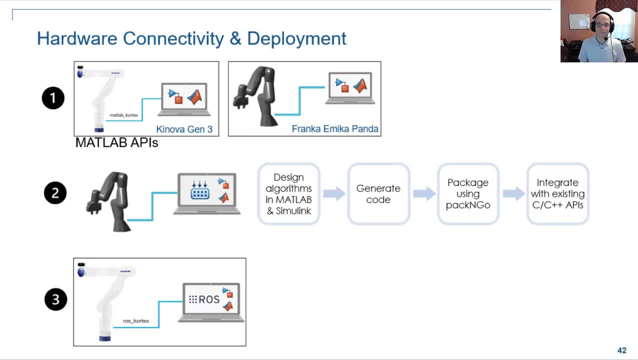 So you can run it on your computer. So if you've just run it on your computer, then the CPU can look like this: have used is connect to ROS right? ROS is a middleware that is a very common interface to many robots and many of the industrial robots are supported by the. 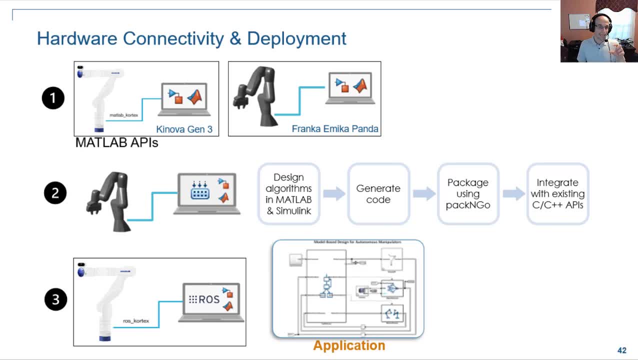 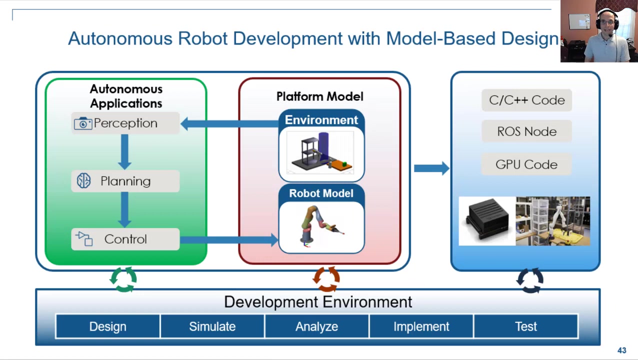 ROS industrial consortium that provide dedicated drivers and interfaces to those robots, And ROS can be can be used to deploy code and it can also be used to communicate to the robot in real time while while it's running. So with that I think we covered the whole cycle and I hope I showed you a little bit that. 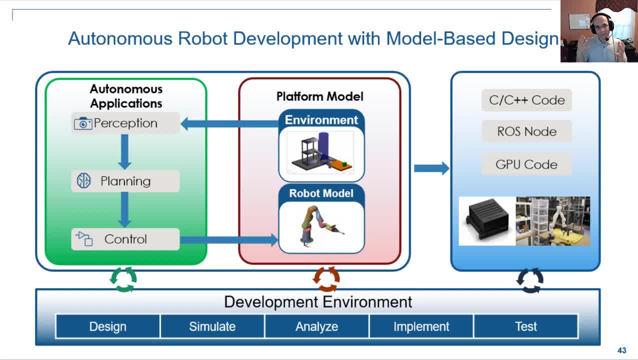 model-based design can be a way to start with a robot model, design your autonomous algorithms and then deploy them to the robot. And again, we have seen success in many of the companies we worked with in using this approach to dealing with more complex smart factory problems and using cobots. 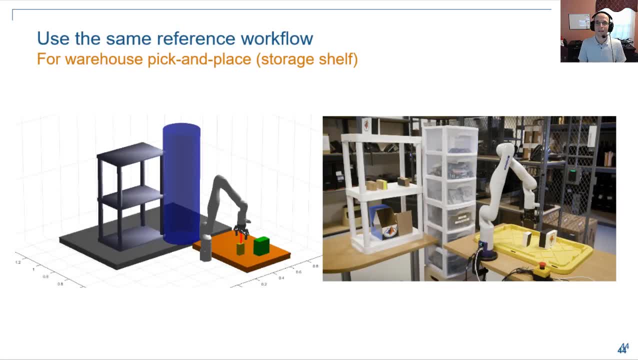 to address those problems. So here are two more examples that have a bit more of a practical setting. So this first one here is for a simple warehouse pick and place application where a robot sorts and detects objects and places them onto shelves. Again, it uses the same methodology that I just 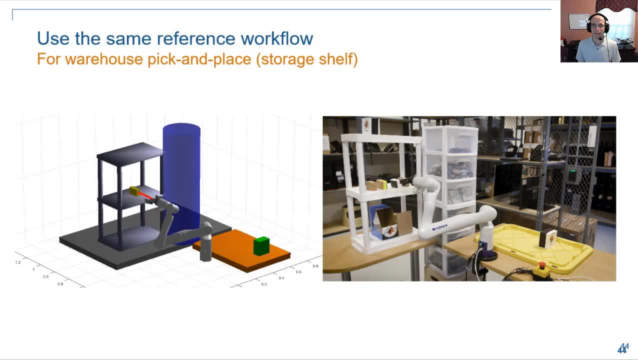 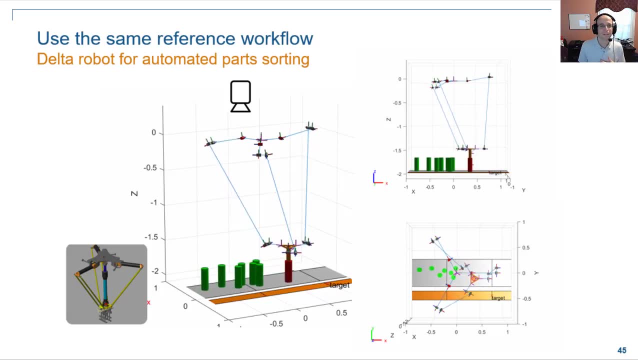 described, but for a slightly more complex application. A lot of companies we've worked with also deal with delta robots, So in this case, here you might place objects on conveyor belt. Again, same principle applies. Different type of platform, different type of planning. your 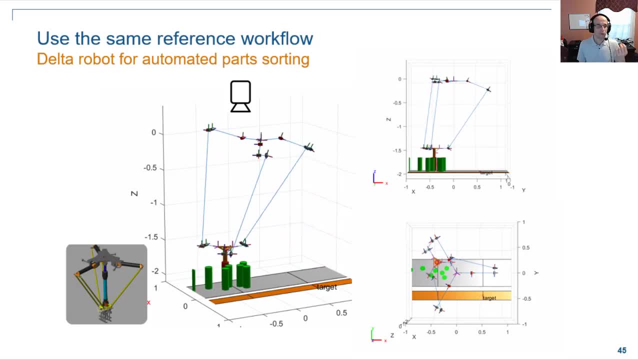 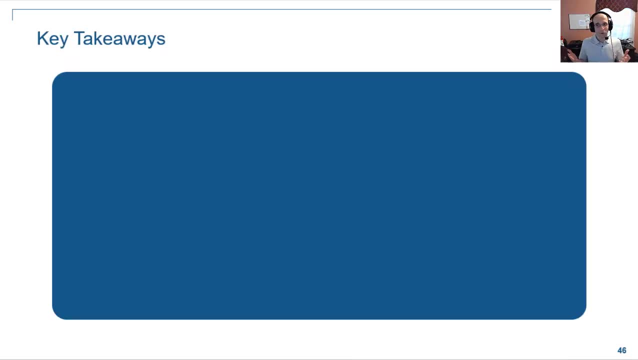 performance, But the same steps, the same modularity applies that I showed you in the earlier workflow steps. So here's a quick recap of what I talked about. So I talked about kind of advanced robotic systems and how they will shape the factory of the future And then talked about kind of the three. 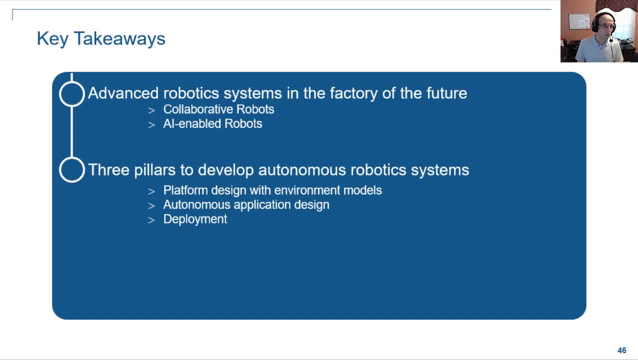 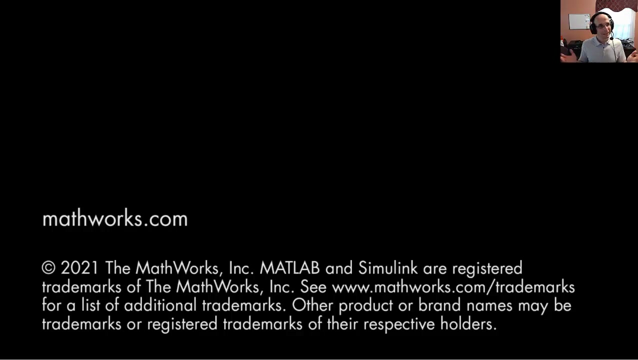 pillars of what we, what I see as important steps for developing reliable, safe and scalable autonomous robotic systems. And you know, I hope you got a flavor of what model-based design is and how it helps in those applications and how it helps our customers deploy those cobots. And with that I want to say thank you and I'm 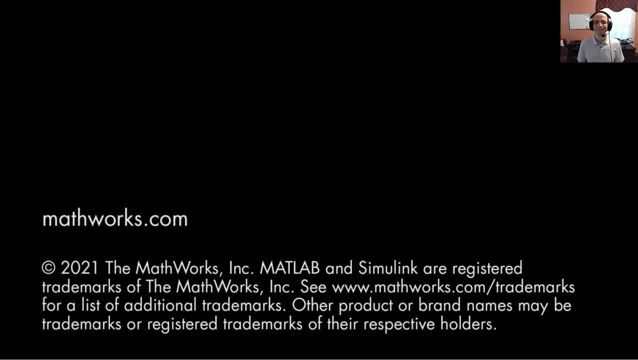 looking forward to your questions in the Q&A.